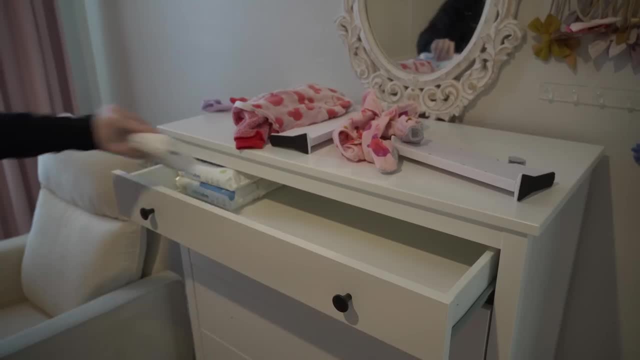 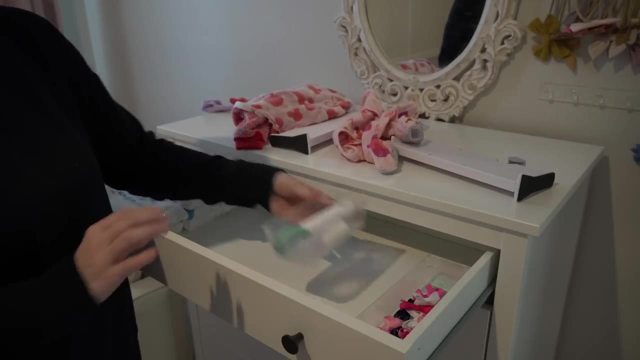 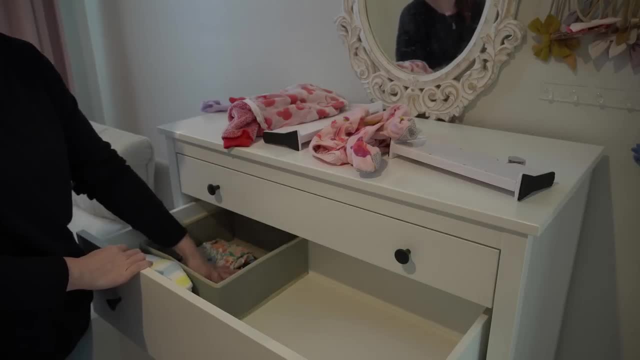 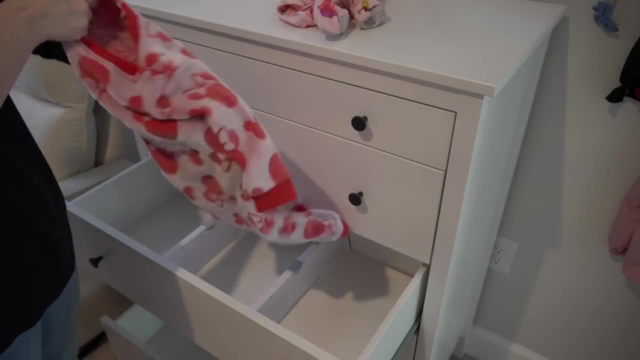 furniture. I love their furniture. I love their furniture. I love their furniture, And this isn't the most expensive one, but I like the quality. It's really really good. I also wanted a taller chest of drawers. That way we could just kind of save space, And I like it. It's really cool. 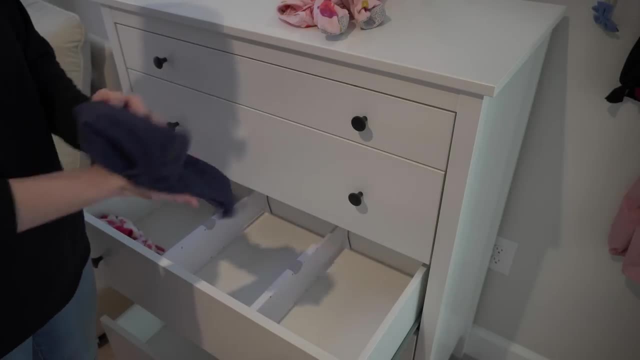 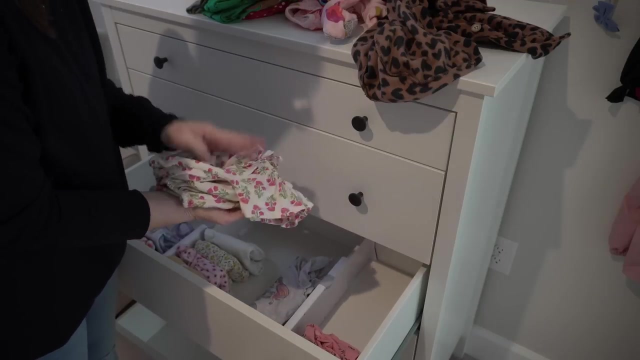 And I don't know. I can't even remember the name to it, but I like it a lot. I also want to add: if you are new here, welcome. I am so glad you're here. I create content of cleaning, decorating, decluttering and organizing as a mom of six. 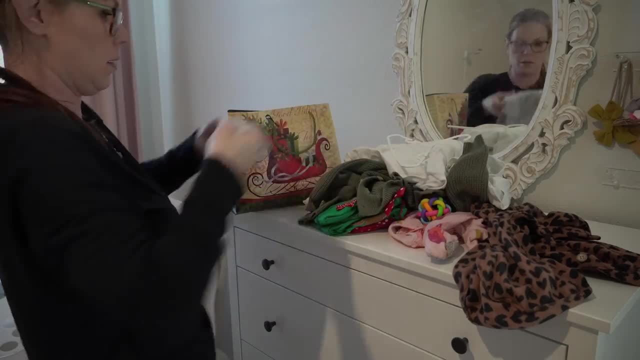 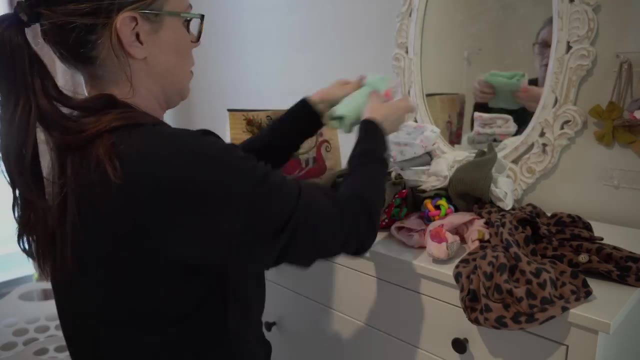 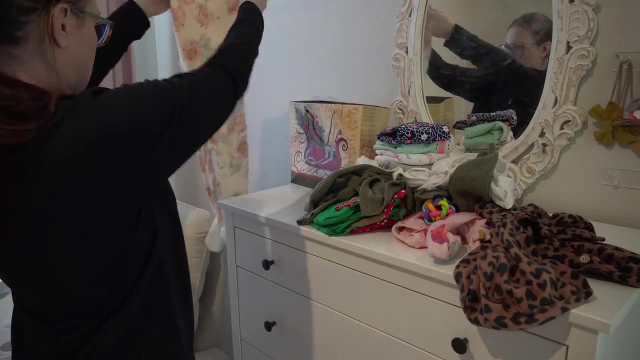 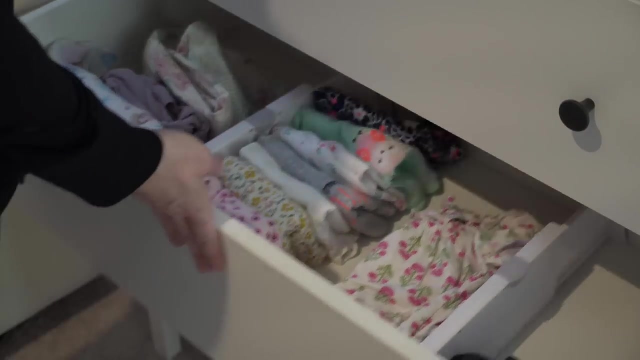 We've always got something to do. So I posted on our community page that I had clothes from one year to 18 months and I had a wonderful foster family pick those up from my porch, which was amazing. This really does help me. 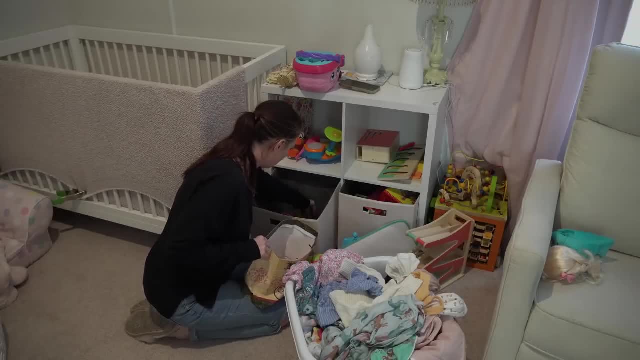 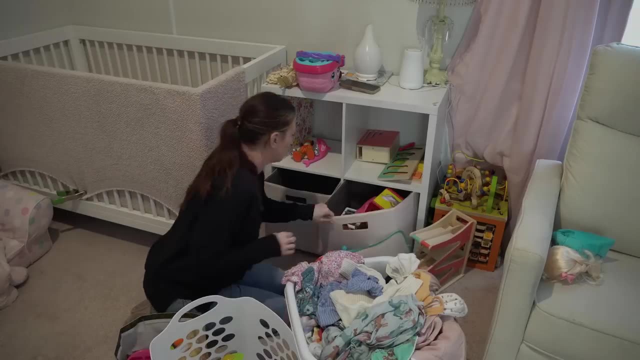 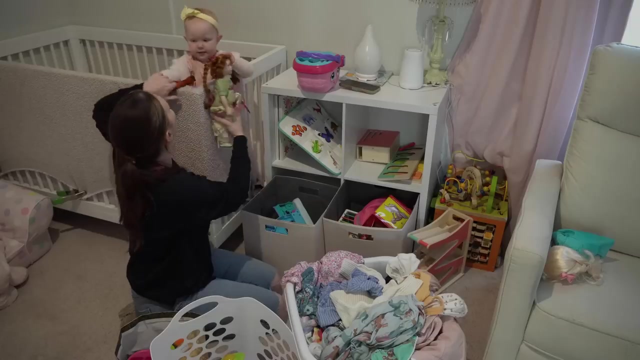 I love to help people. I love to help people in general, But when you are maybe getting rid of stuff and it's hard for you, just remember how you can bless someone else. Just put on your community page or Facebook Marketplace free and I'm telling you it'll be out of your house really quickly and it'll save you a trip. 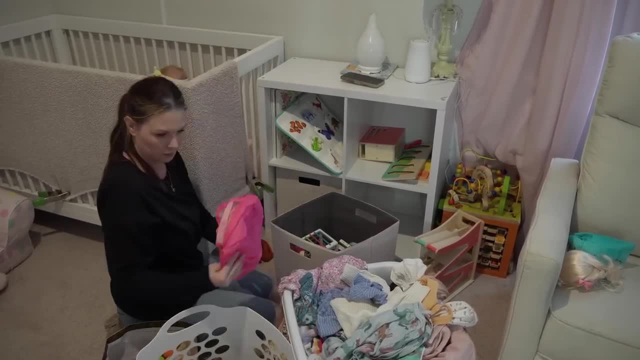 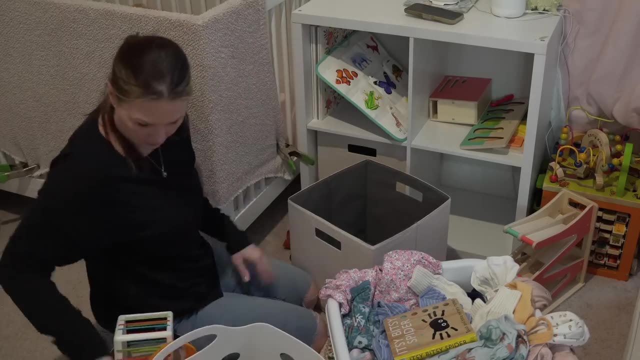 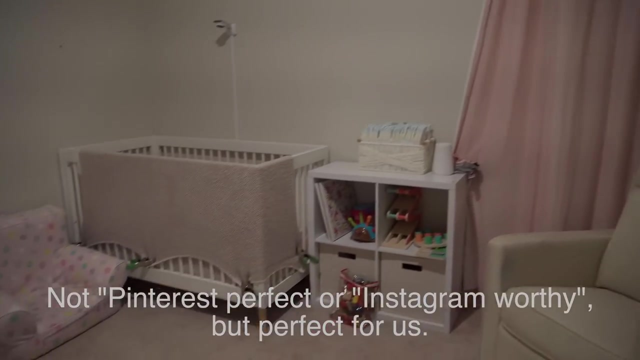 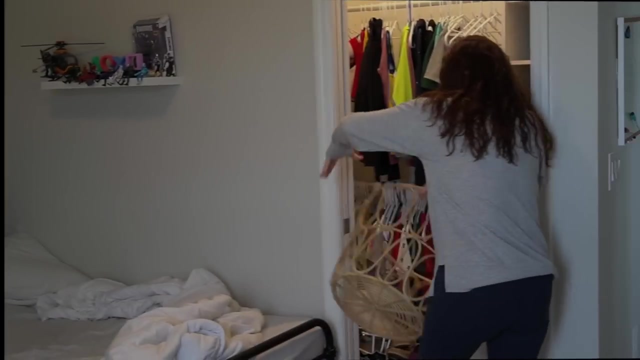 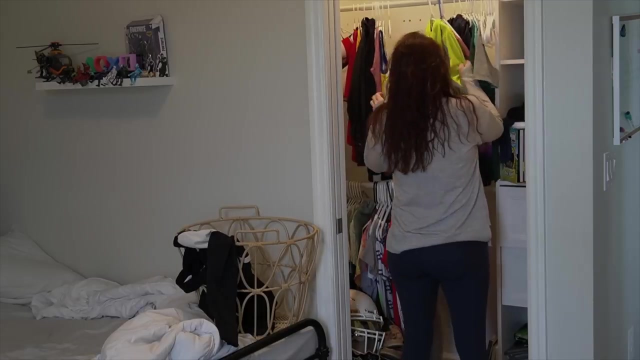 I did the same thing with the other dresser and the changing pad, So this was all gone and I didn't have to lug it around, But, more importantly, it blessed another family. Okay, we are in my boy's room. This is my eight-year old and my 11 year old. Sorry, 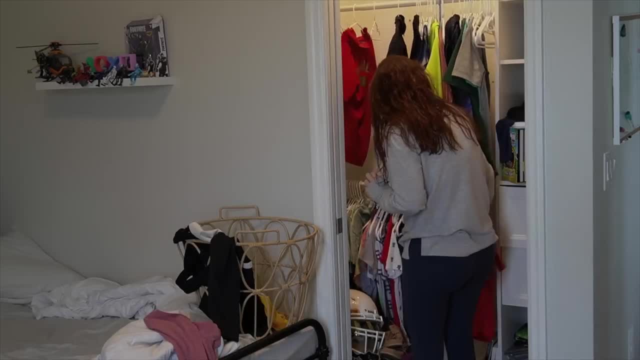 I had to think about that And my eight-year-old will be nine in April. This is Noah and Josiah's shared room And I wanted to come in here because I knew the kids and they were going to stay in this room. So I made a reservation for these four-star rooms and I'm going to show you what they're all like. 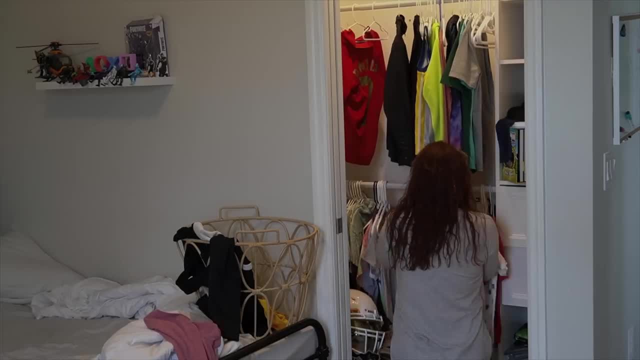 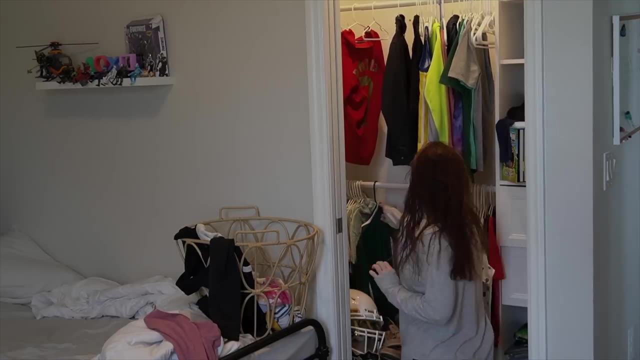 And it's going to be an amazing experience. So I'm going to show you what I'm thinking right now. knew this room needed to be decluttered, like something crazy. I always come in here and I'm stepping over clothes and there is so much laundry to be done. constantly There's just stuff thrown. 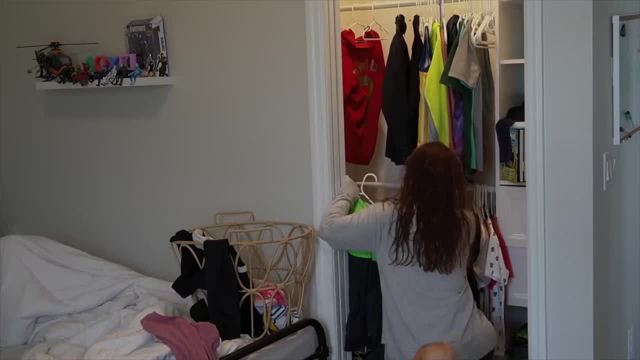 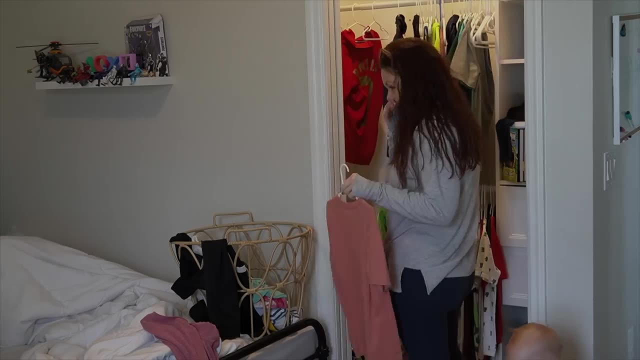 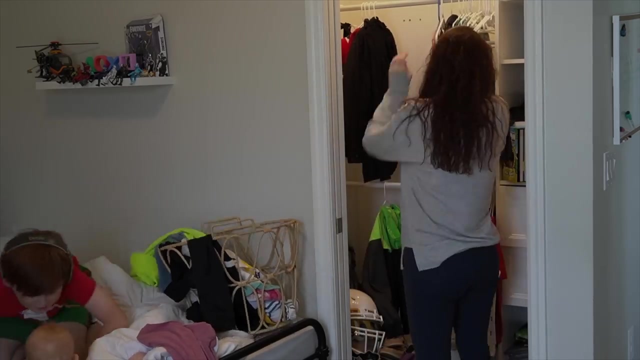 around and I was over it And I know for myself and for my children that we do better in open spaces, uncluttered spaces. So I wanted to tackle this. I've been putting it off for probably a year now, And today was the day. I just wanted to get in here and just knock it out, And that's what I've. 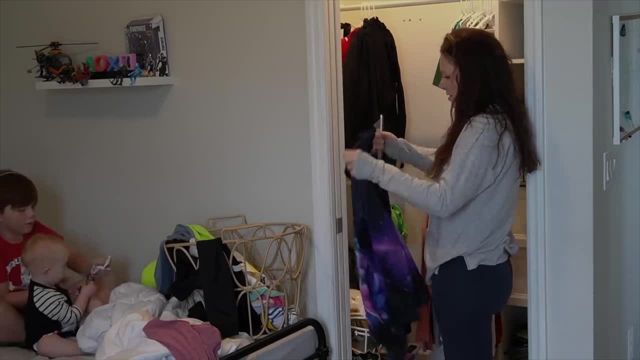 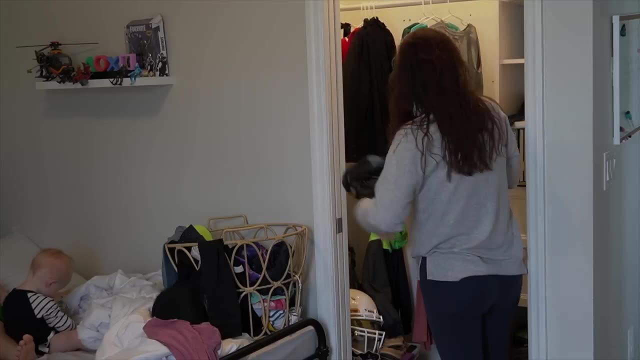 been doing with all the areas of my house where I'm like I just been putting it off, like the big areas that overwhelm me. I'm just getting in there and just knocking it out And it feels so good. When I show you the before and after, it's pretty crazy, But to tell you that I was able to actually 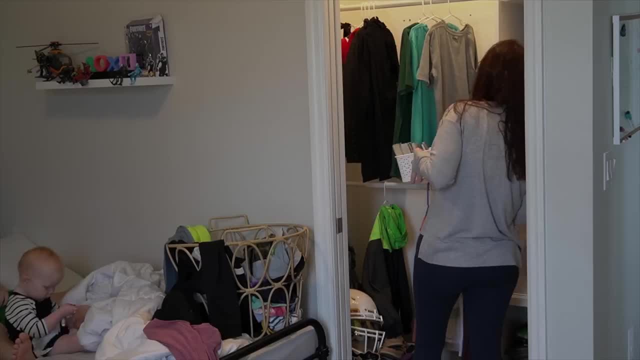 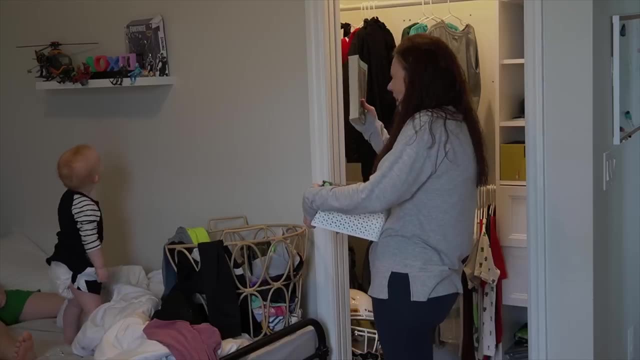 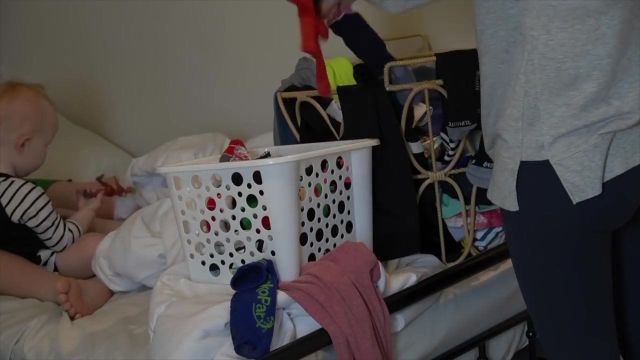 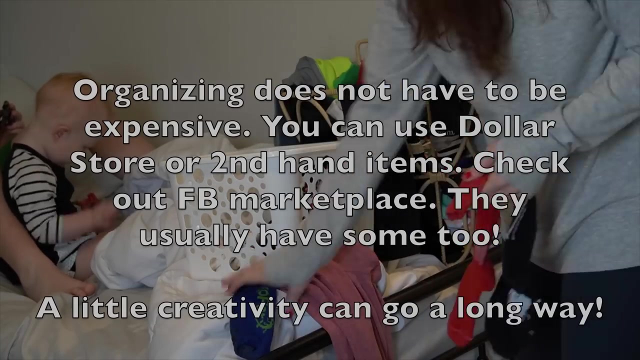 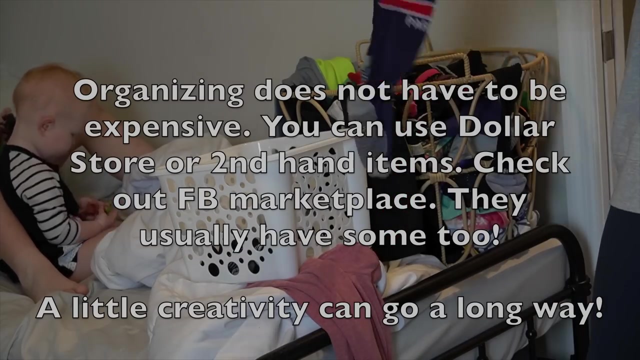 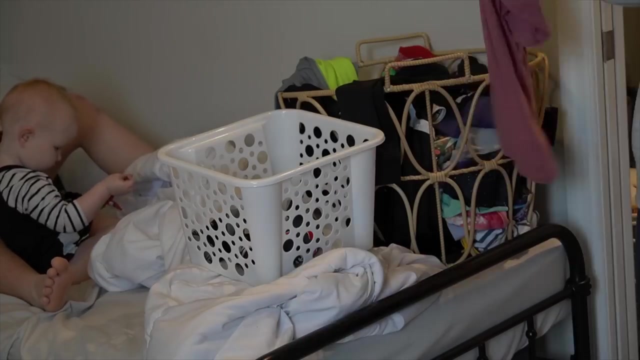 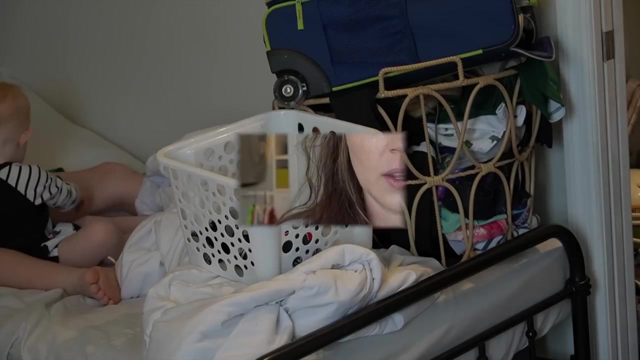 take a whole carload. my truck was full to the brim of things I brought out of here. It shocked me so, so much. I could not believe how much I was able to get rid of. Okay. So when I'm going through things and decluttering, I can go very quickly, Like the. 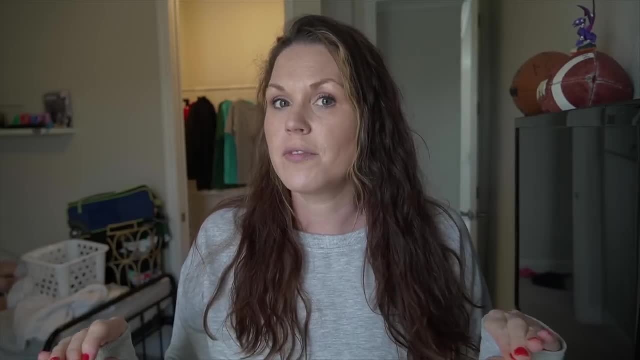 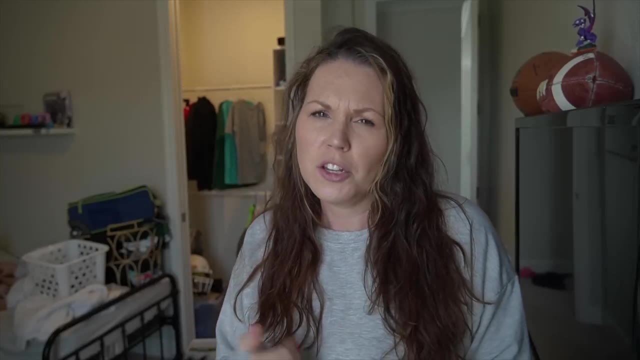 first pass. I can be really quick: Just go through there. Whatever I just know right off the bat that we don't need, I'm going to put it in the basket. When it comes to the kids stuff- clothes- I can usually do myself Toys and like things like that- I do like to have them involved just high as 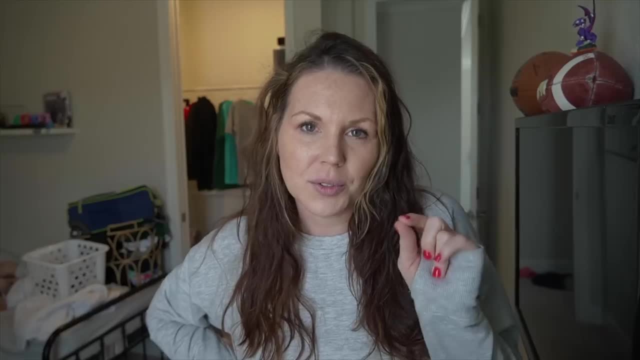 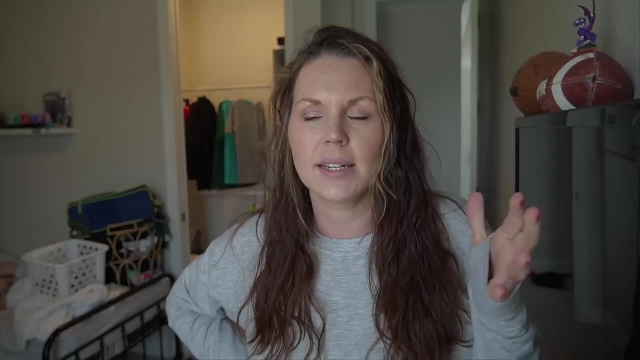 high as I can. So I'm going to take that into consideration when I'm going through their items. So that made it a little bit easier. But I also know the things that I wash repeatedly and the things that have been hanging in their closet for a really long time. So I take that into. 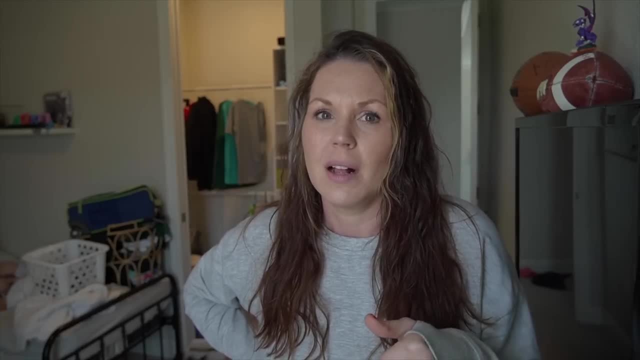 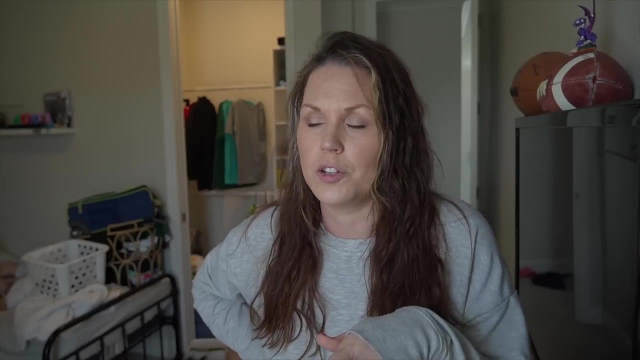 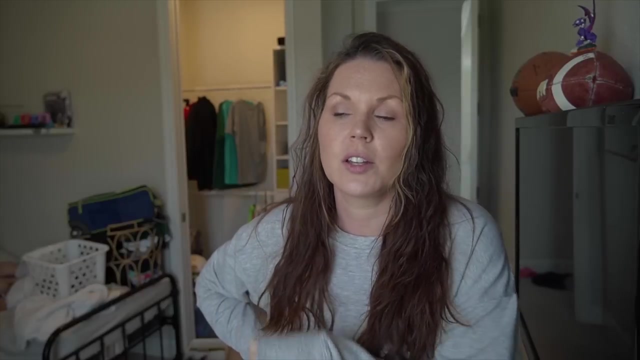 consideration when I'm going through their items. Also, I don't love laundry. They don't love laundry. We have way too much stuff Like it's just way too much And honestly, those are the things that really overwhelm me And I don't. they don't know any differently. So, going through all 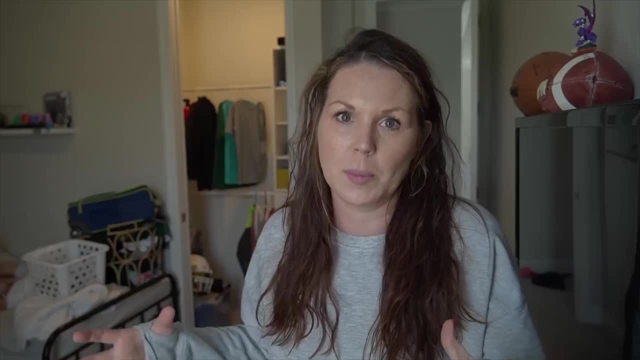 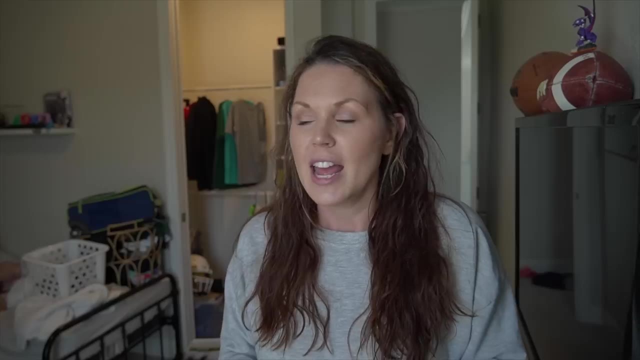 these things. it might seem like a big thing and they're going to see all these open spaces. It might kind of be shocking at first, but when you get into the flow of it it will feel so much better, Not just look better, but it's going to feel better. I can't really explain it until you. 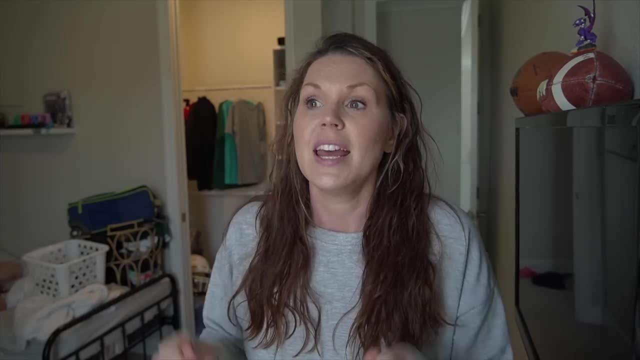 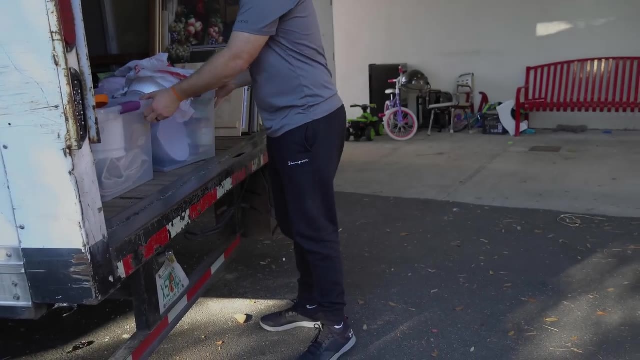 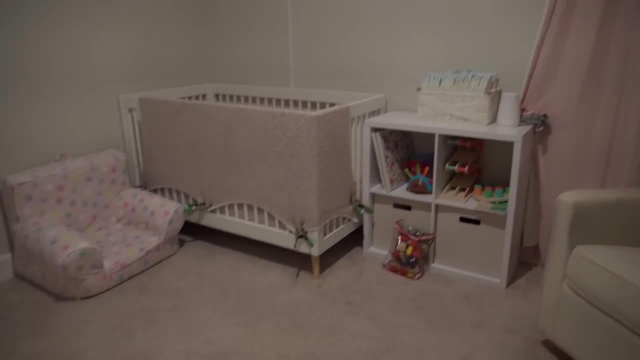 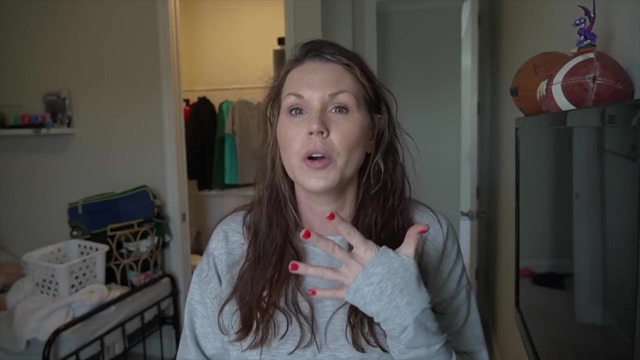 So it's just so much: more room to make, more memories, your imagination to flow. I'm telling you, removing stuff from your home that you no longer need or no longer bring you joy or serve you. it's more than just decluttering, It's more than just donating to families in need. It is about 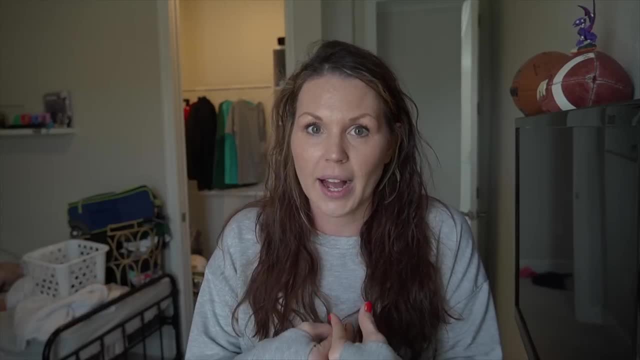 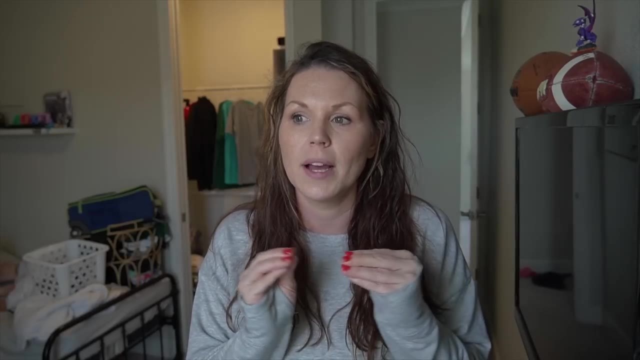 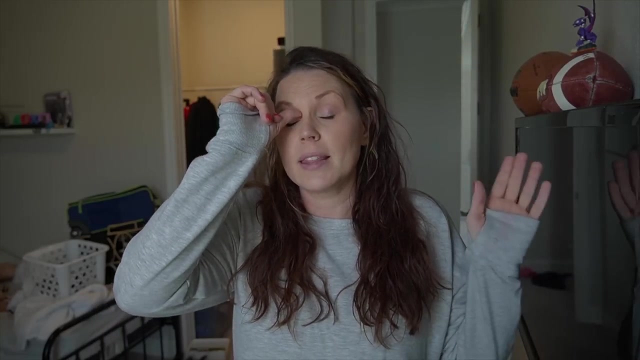 literally opening up space where you can thrive and you can grow and you can literally just be your best self. I cannot explain to you how much it will change your life by decluttering a little space in a little drawer, closet your room, whatever Big, big things or small things, it will literally. 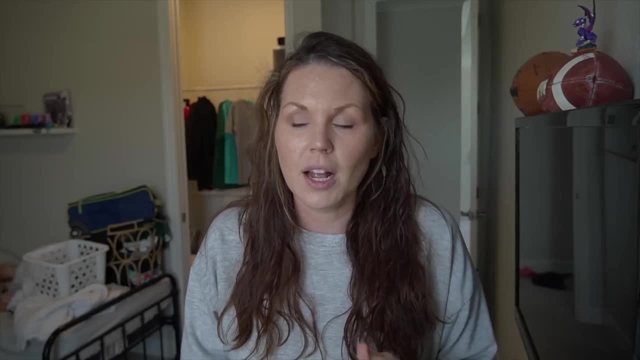 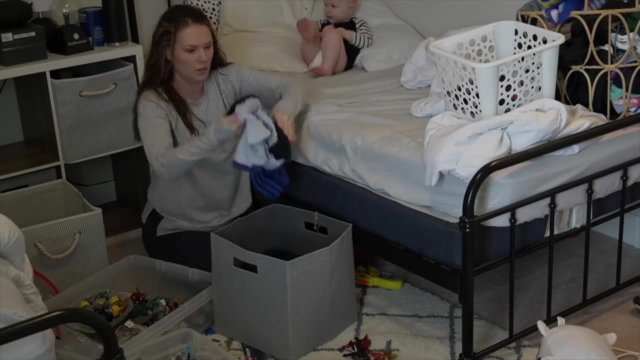 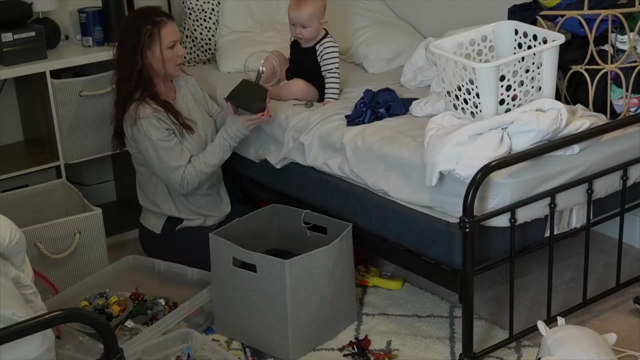 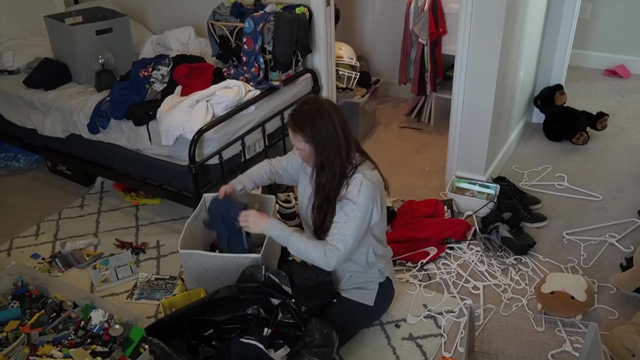 change your life and it will start setting in motion more decluttering and getting control over your spaces. So I've already done the big sweep of their clothes. I am now going into the little cube organizer and these little containers here and getting more items out. I'm filling up. 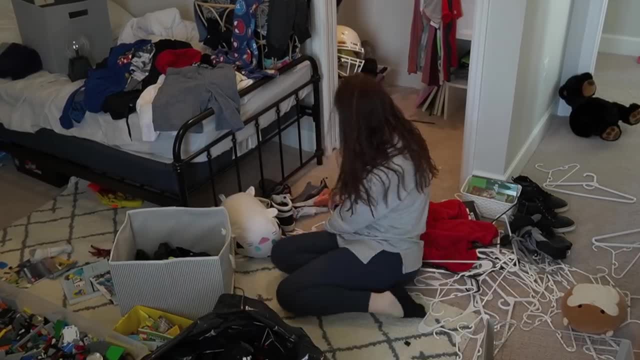 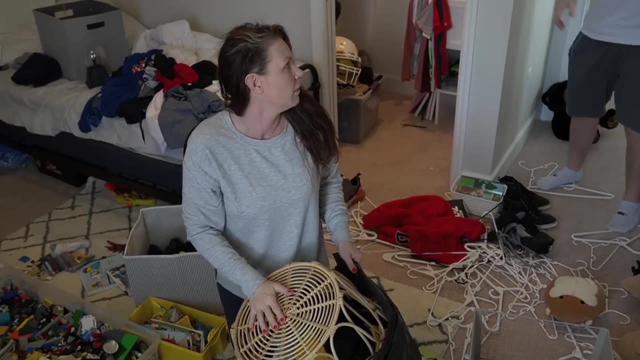 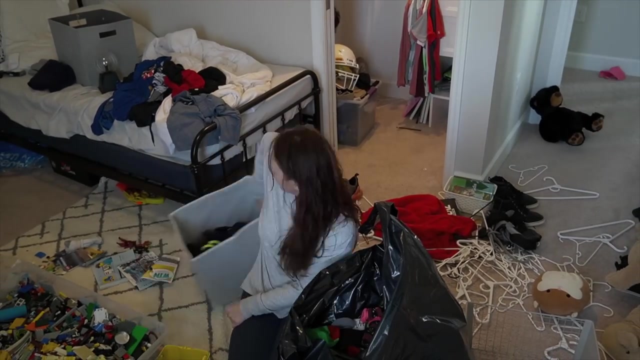 this black trash bag. Now here's a little tip that I would like to recommend to you guys. You can definitely go in there with like regular trash bags, but in my opinion, you're better off doing a black trash bag or even a box- not a clear box, but a box- Because if you're anything like me, 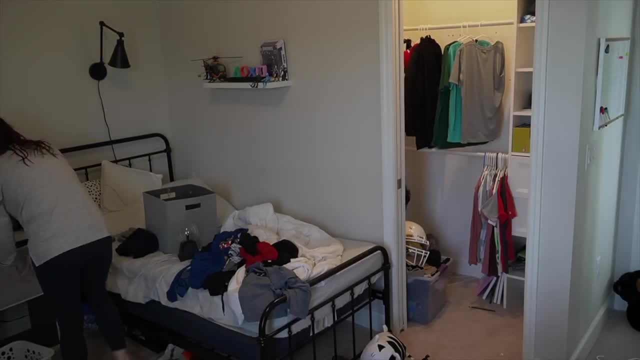 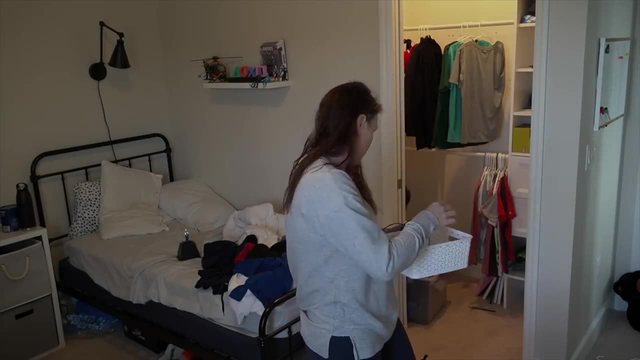 when I started this journey, I would go back into the items that I decluttered and got out of the space and I would bring them back into them. I would see it and be like, oh, actually, I really do like that, I think I'm going to take it back And I would do that. But if I use something that 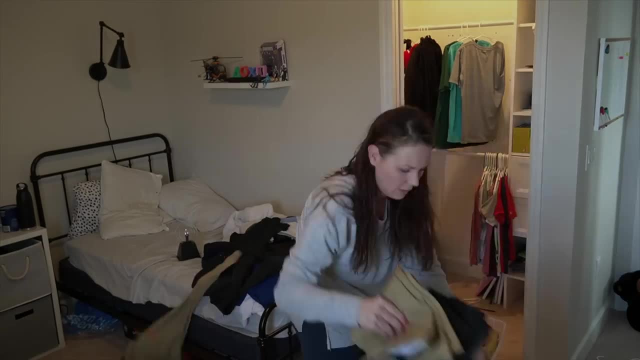 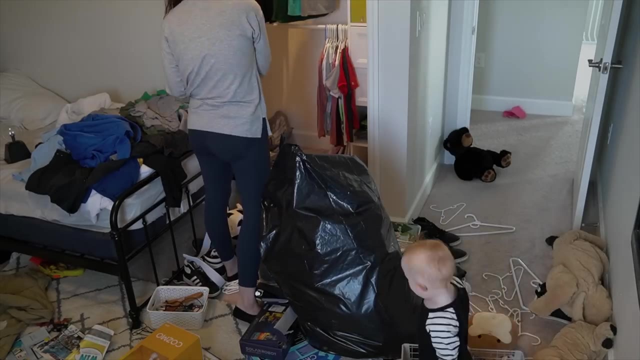 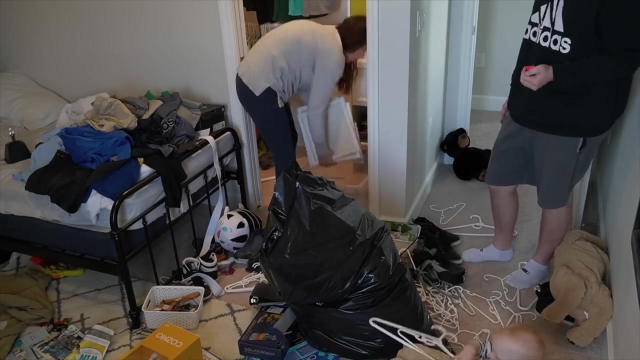 I cannot see through like a black trash bag or a box. I don't see those items and they are gone. They're out of my sight. I will put it in the garage or my closet or set it aside, And I do not fumble back in there at all. Once it's in the bag, it stays in the bag and take it from me. 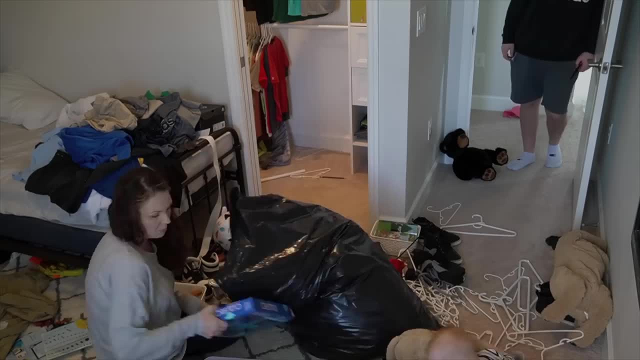 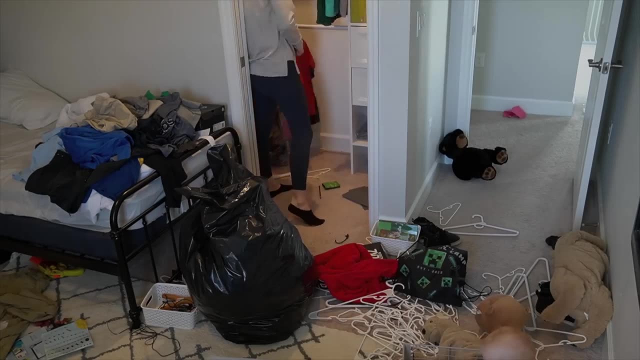 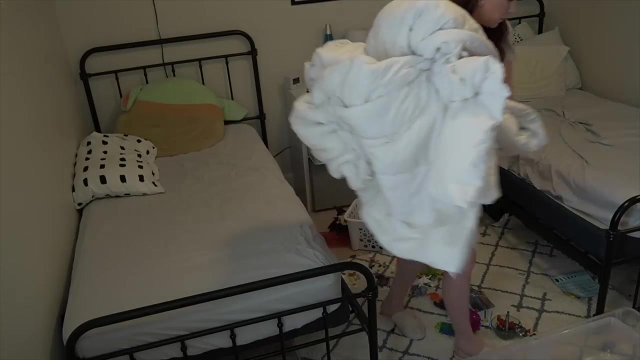 It took me a long, long time to really get comfortable with this step, But having something that I cannot see through really really helped me. It just kind of helps. you just not see it. If you don't see it, you don't think about it, And then you realize I didn't need it all along. So I'm in the room now. 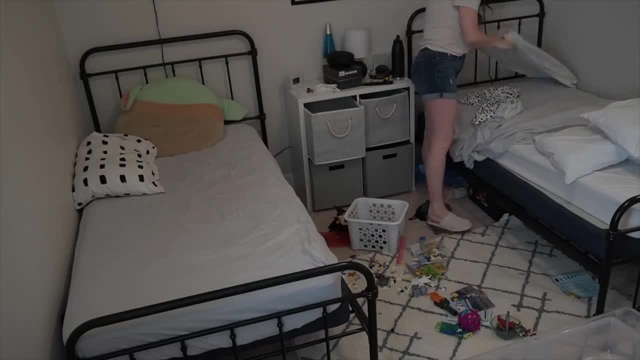 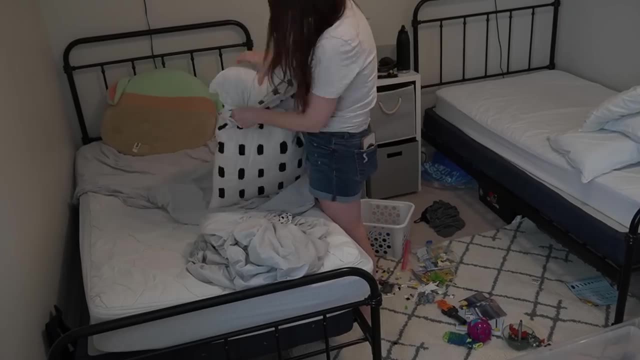 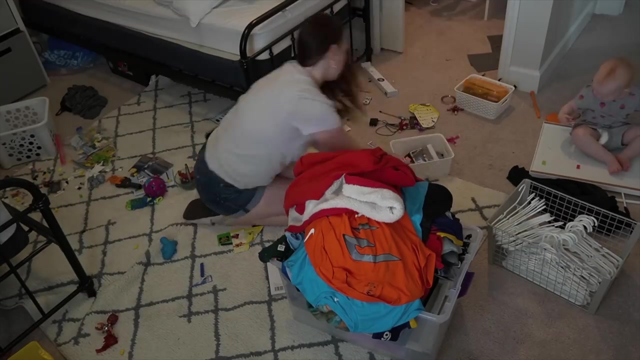 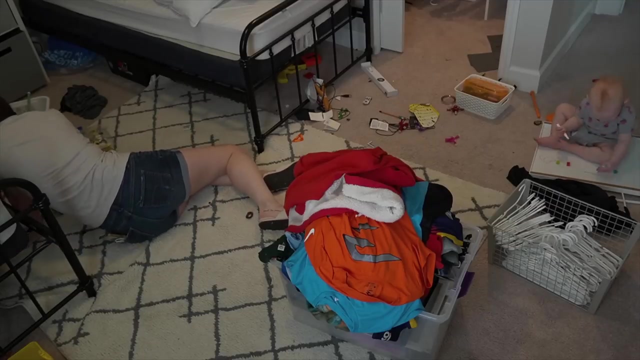 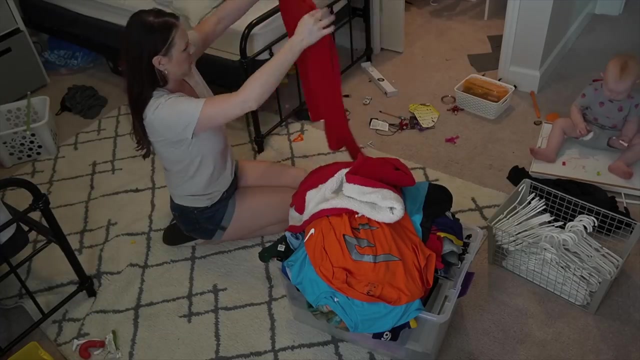 I've done a huge sweep- huge- And I'm going to clean their sheets really quick. I'm just going to zoom through here. I'm going to throw these down over the banister and start washing them as I continue to finish. So the boys had a ton of Legos and they were being stored underneath the bed. Well, I did post. 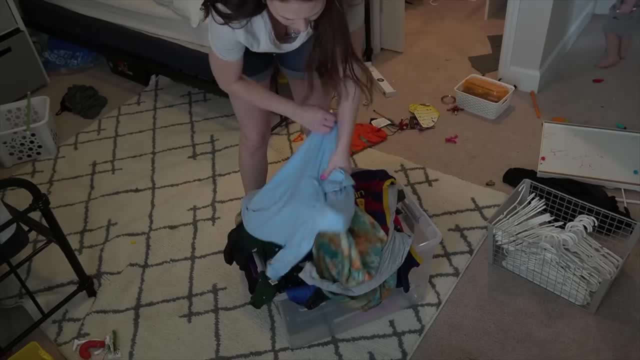 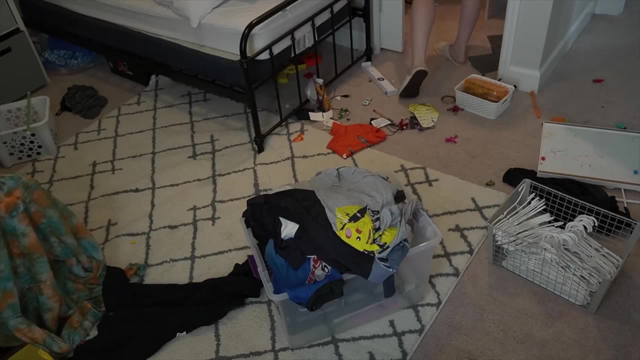 them on Facebook Marketplace for a hundred dollars. They weren't selling, So I was able to get a buyer for 40 bucks, which I didn't mind because they were really heavy. I didn't know what else to do with them And they're going to go to someone in need, which is totally fine with. 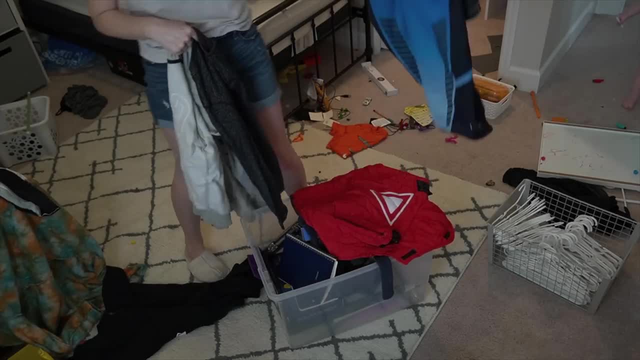 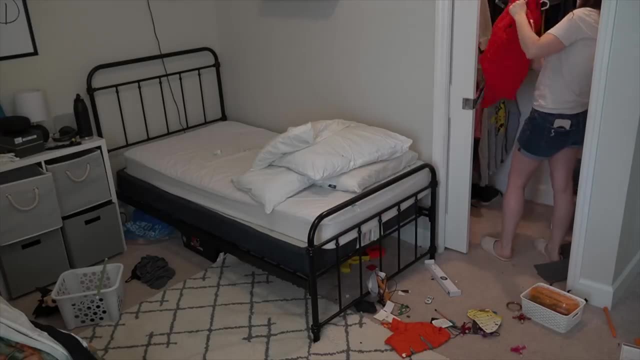 me, Then I'm going to go through all of their clothes here. I'm going to hang some things up. I've got to get them some different hangers And I'm just going to go through here really quick. Now I do want to recommend: when you are decluttering, I always tell you guys to start off. 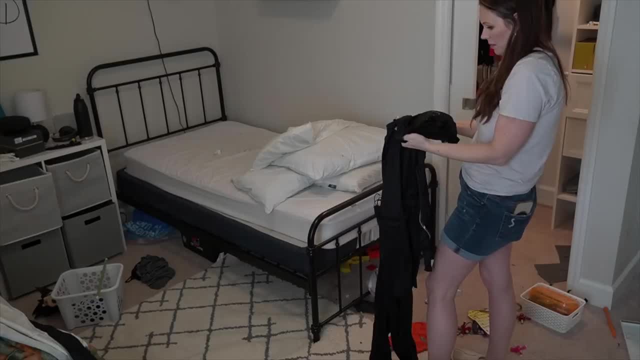 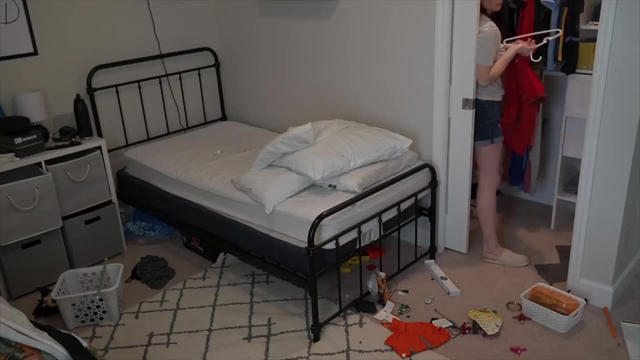 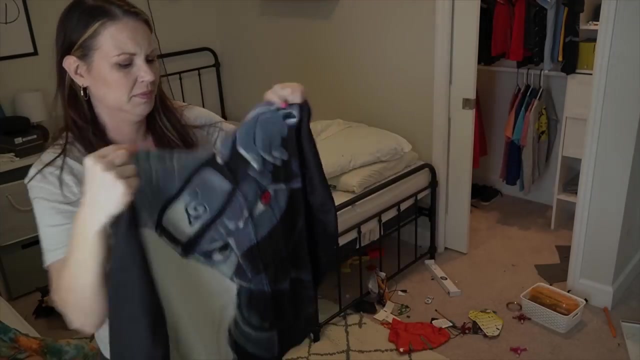 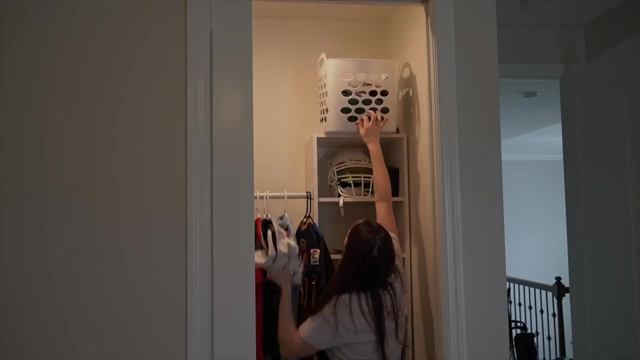 with trash. first and foremost because it's easy. You want to start easy, especially if you are just getting into this. It just helps you set the momentum And then you can do more and more things. So this is a jacket that Noah loves- Not my style, not my taste. I don't want it in the house. 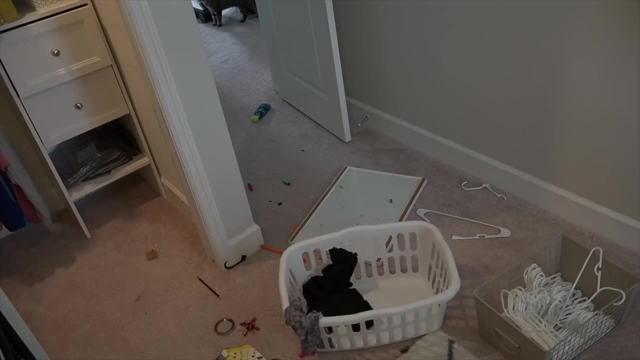 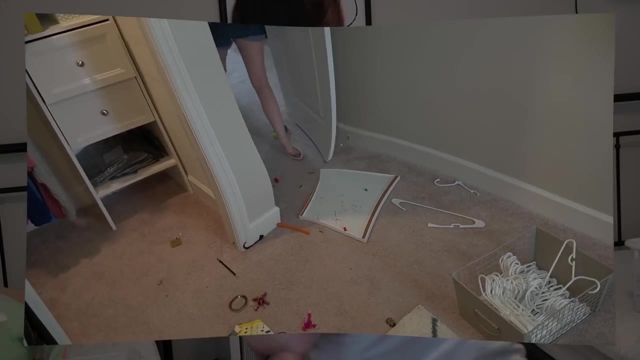 but he loves it. However, it is way too big for him, So I'm going to place it in this bin right here, because I know how much he loves it And I think it would be really, I don't know, disrespectful, I don't know how to say. it Just wouldn't be very nice to just throw something. 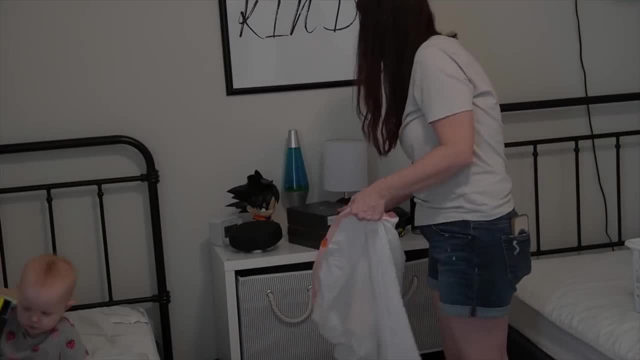 out there. I don't know how to say it. I don't know how to say it. I don't know how to say it Because it isn't my taste. I won't do that, So I'm going to put it in that bin. and when it will? 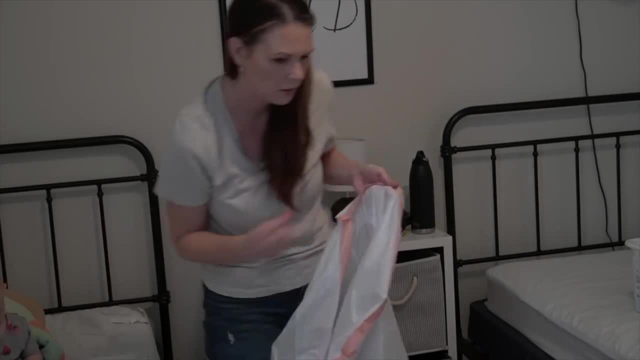 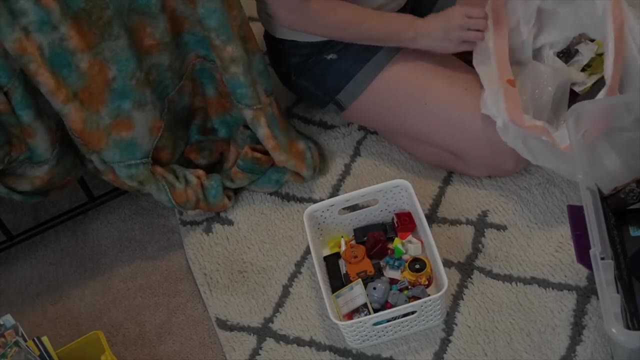 fit him. he can then decide if he wants to keep it any longer, But that is what I do. There are some things that I don't like, and it doesn't matter if I like it or not, because they love them, And that's what it's about. So I try to definitely respect their boundaries and their 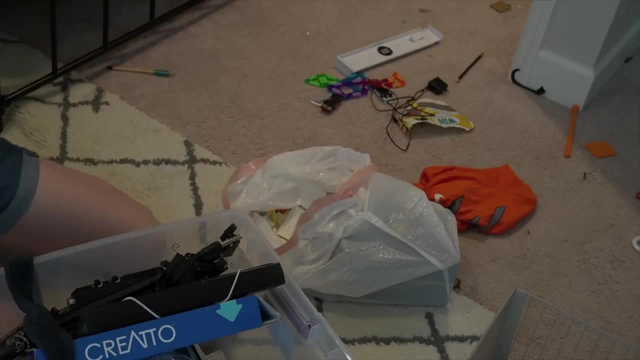 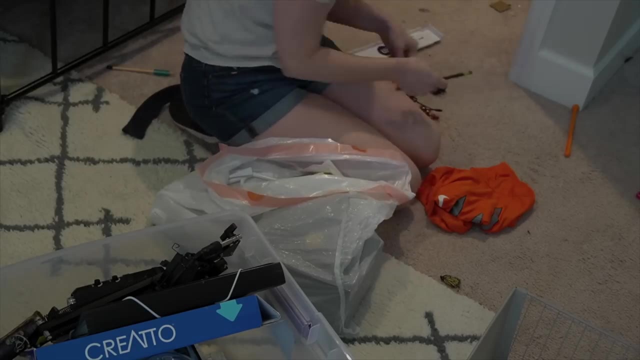 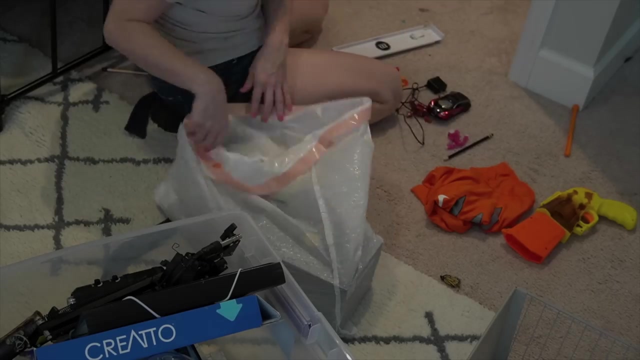 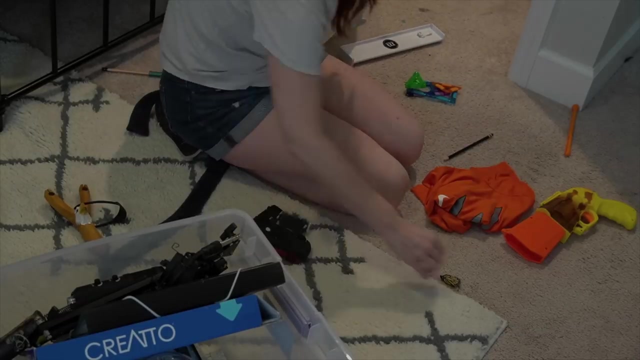 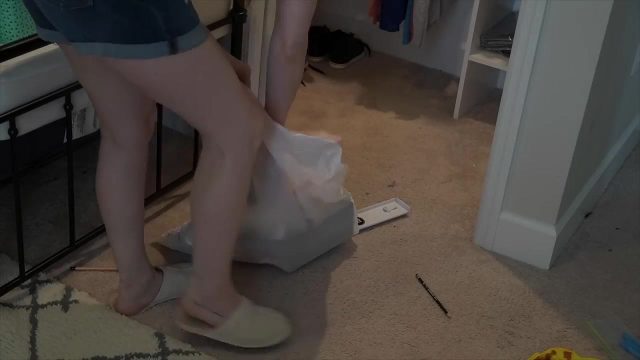 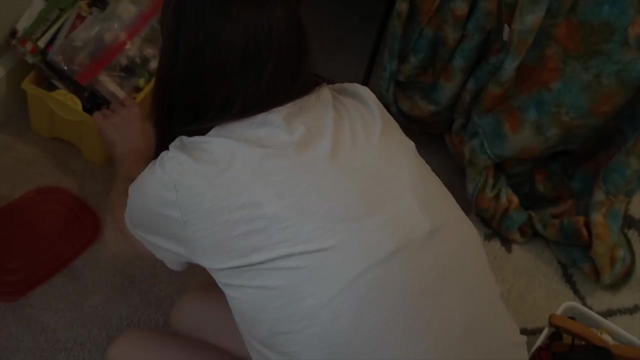 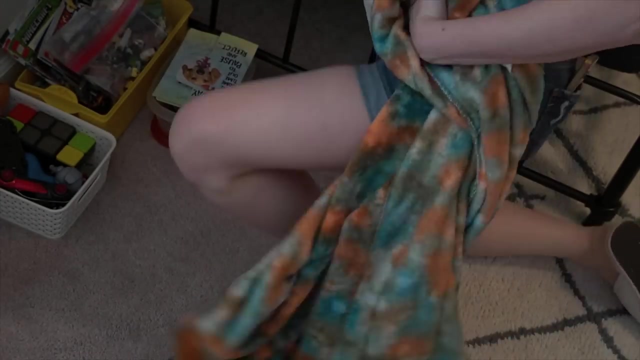 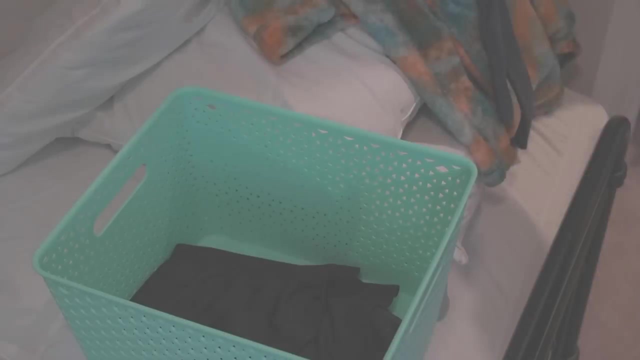 items when I go through this process. So I try to respect their boundaries and their items when I go through this process. So I try to respect their boundaries and their items when I go through this process. So this little bin here I'm going to put their costumes in. Noah still likes to dress up in his 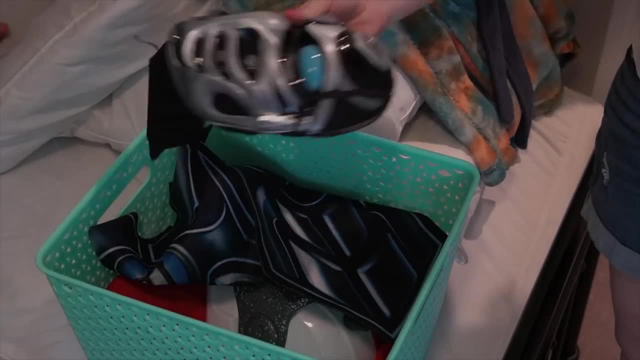 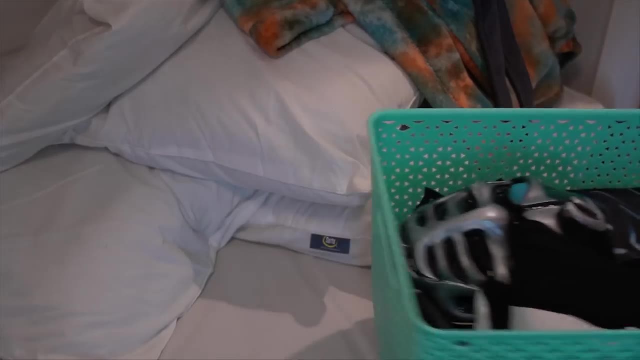 Halloween costumes, which is so cute to me. So I'm going to make a little bin here for him that he can go and get the stuff he wants and surprise me in his little skeleton outfit at any time that he chooses to. So it's cute. I love it. 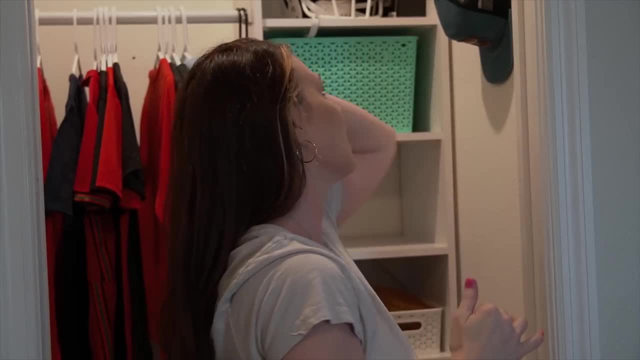 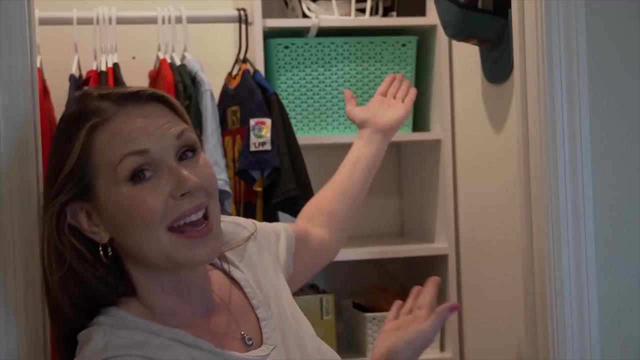 So I have an idea. We've got these extra pushpins over here and it just dawned on me as I was looking for a place for their hats. I'm going to use the pushpins. It's minimal damage and it hangs their hats perfectly And it gets them off. Hold on, baby, I will. It gets them off. 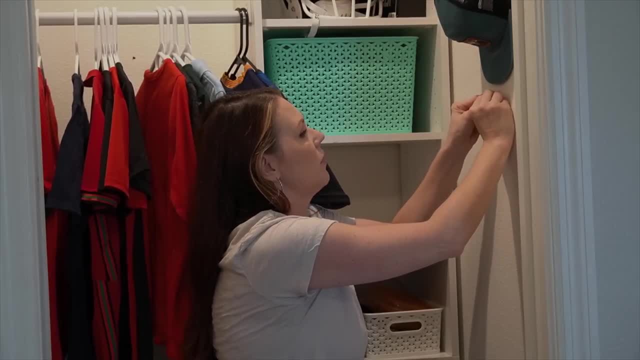 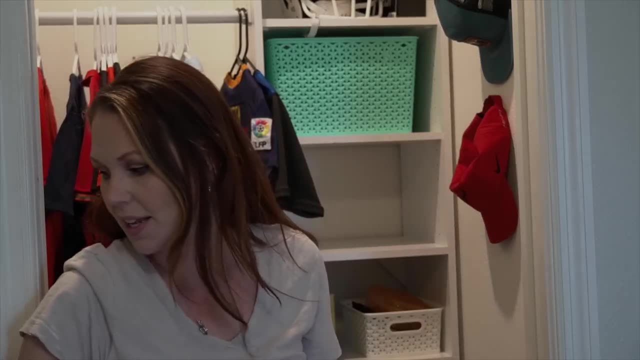 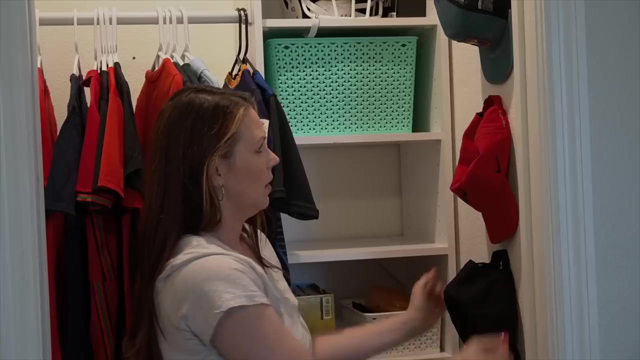 of the wall Or, excuse me, it gets them off of the floor. Get some off of the wall Or, excuse me, it gets them off of the floor. Perfect, You got to just think outside the box. Perfect, Ta-da, Perfect, And it didn't. 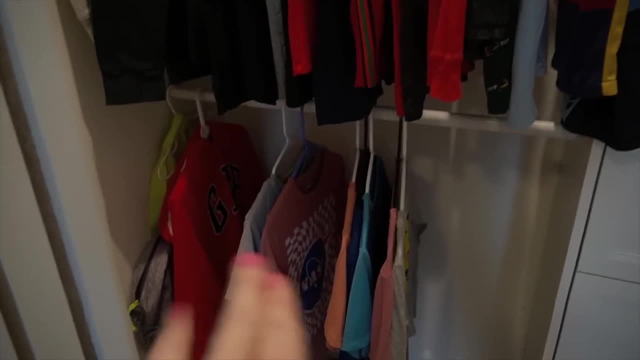 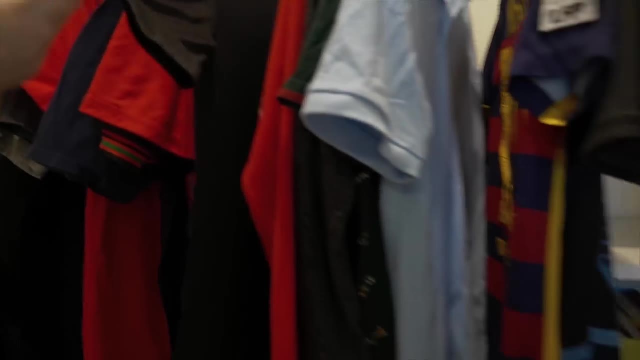 cost a dime, So that always makes me really happy. So here are Noah's clothes. Minimal Josiah seems to have a little bit more. That's because if you look at him it's wood. That's because because he has a lot of these, because he has tennis practice. but Noah wears those too, and he 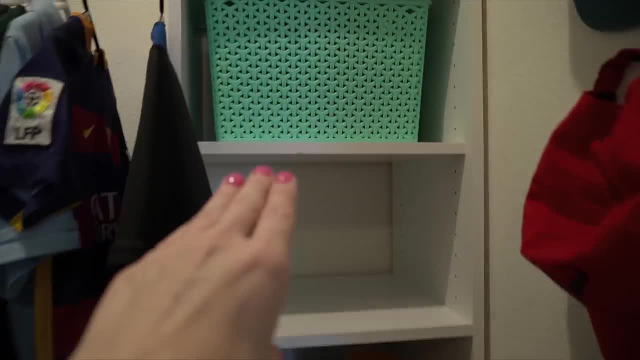 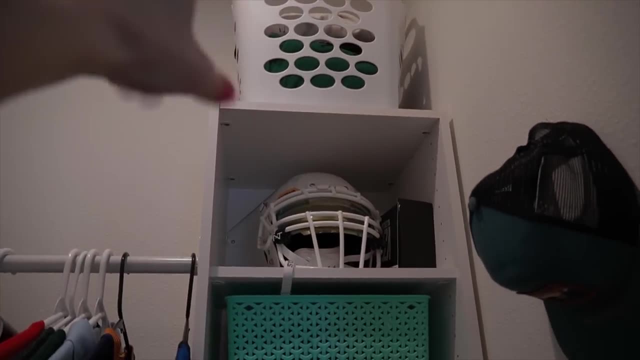 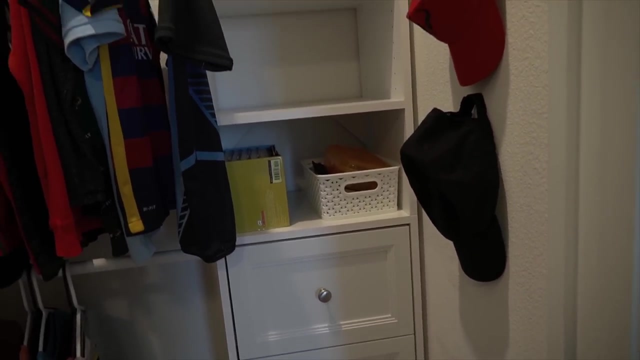 also likes this kind of stuff, and I've got Halloween costumes up here. his helmet- his football coach gave him that these are clothes that don't quite fit, that I know that they can wear. I got rid of a ton that I've been holding since Drew was itty-bitty. he's 17 now, so it was. 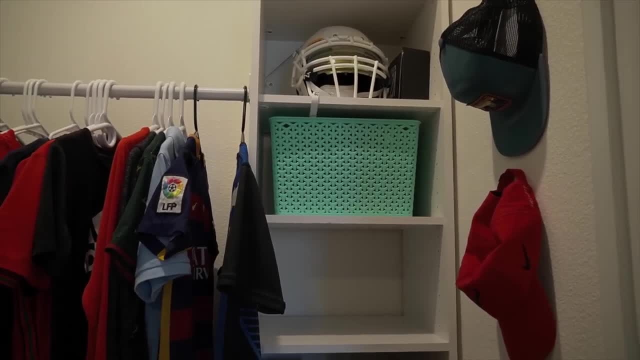 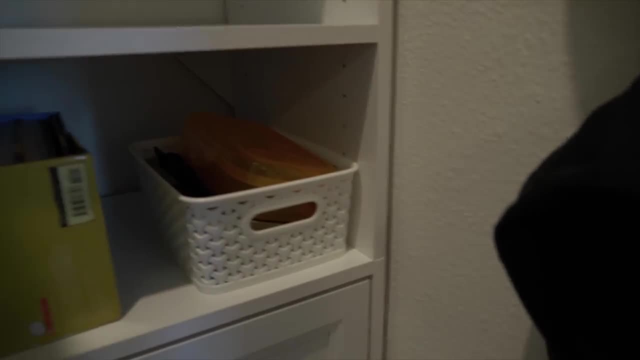 time to let a lot of those go. sorry, I heard something downstairs. I got some staple pieces up there and then this here has got some books. I'm going to go through this with Josiah. I'm going to put it in the pile. actually, I'm going to do that right now. I'm going to put this in the 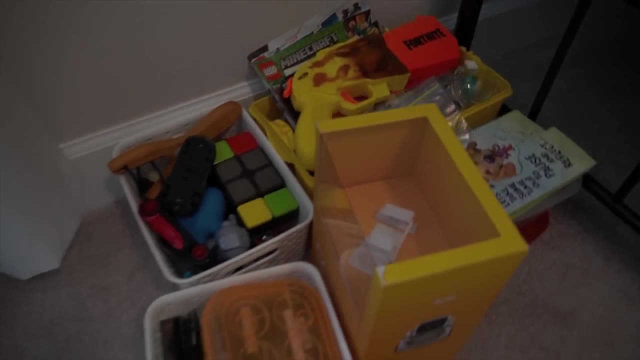 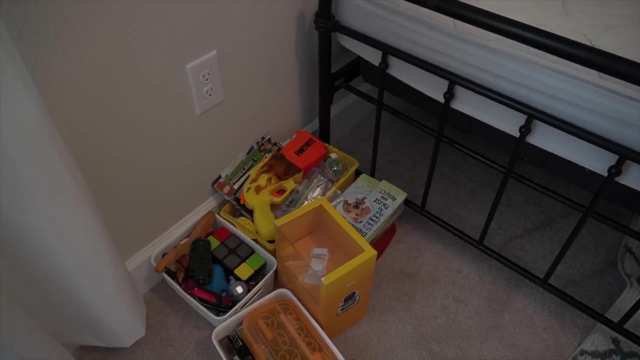 pile. so when it comes to decluttering, I never want my family to think, oh, you know, mom's just going to get rid of all of our stuff. that's not the purpose here. I just want them to learn that. 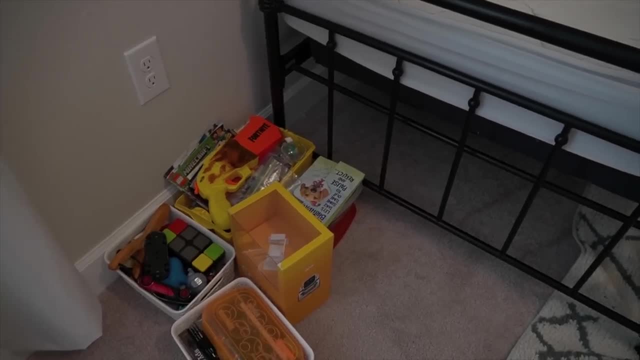 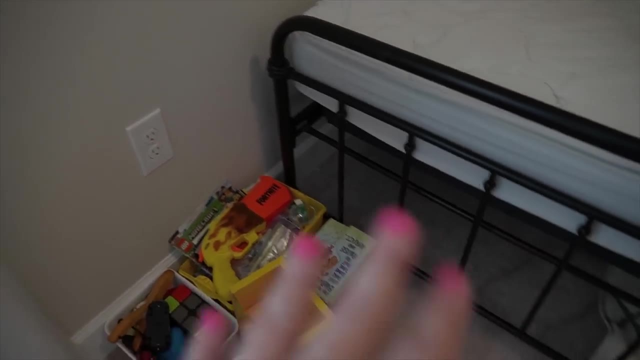 when we have too much stuff, we can't value any of our stuff. so let's just, you know, minimize that so we can really appreciate the things we have. so here are the items. I did sell that giant bin of Legos and so I've got some loose ends right here. you hear Emma singing. 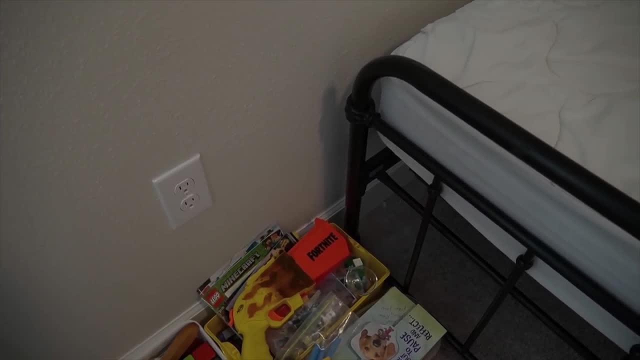 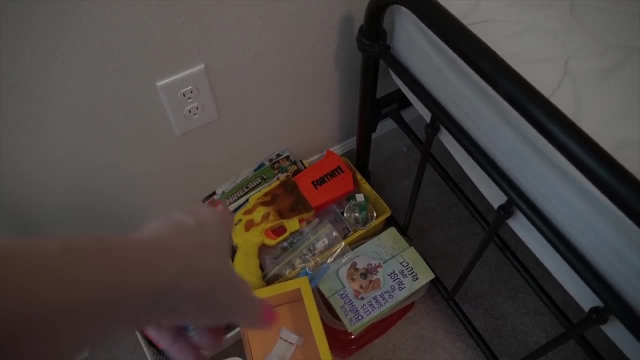 this is the rest of the. I told Noah to come get your favorite Legos before they sell. so these are them. and then I found more, so I put them all here. they're: Fortnite dart thingy, some little odds of Ann's birthday card, a box to his little Cosmo. 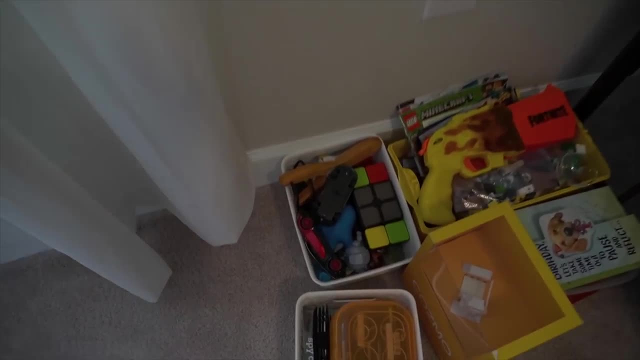 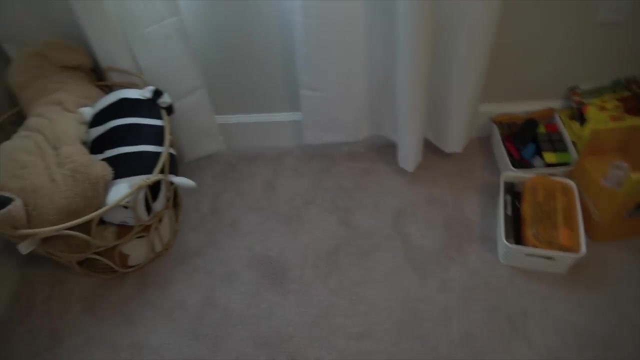 thing, some books and pens, and then some like miscellaneous, like toys, so when they get home from school today also this stuffed animals, things like this I will not just go through and get rid of if it's broken. I pretty much will, unless I've 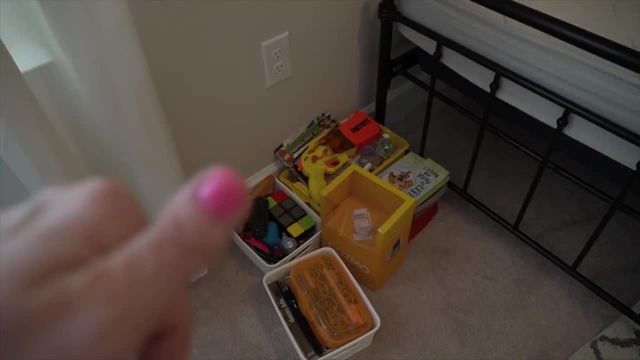 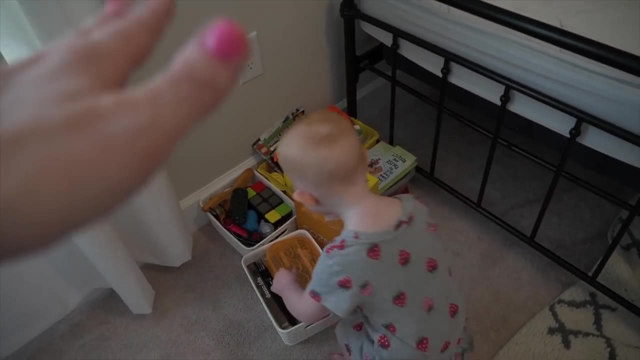 seen them gravitate toward it a lot. then I'll wait and we'll talk through it. but if they're not here, I will put it in a pile, we'll go through it together and we'll be able to go through this quickly. so you'll see that in a little bit. and same thing with stuffed animals. 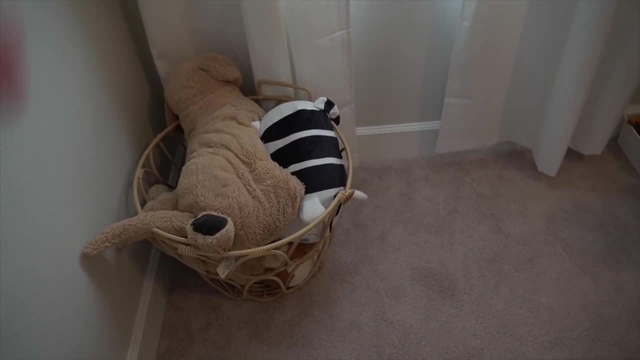 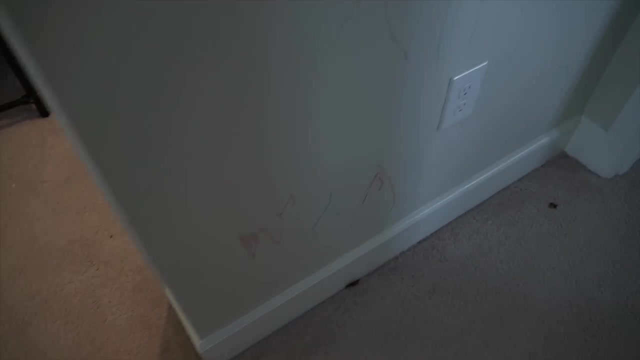 stuffed animals usually have more of a sentimental value, so I like to really talk through thing too. you want to open? well, no, because you've already written all over my walls, so no, we're not gonna do that. here are some items they've had in their 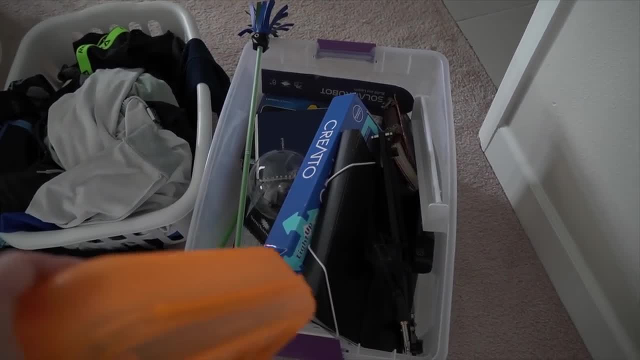 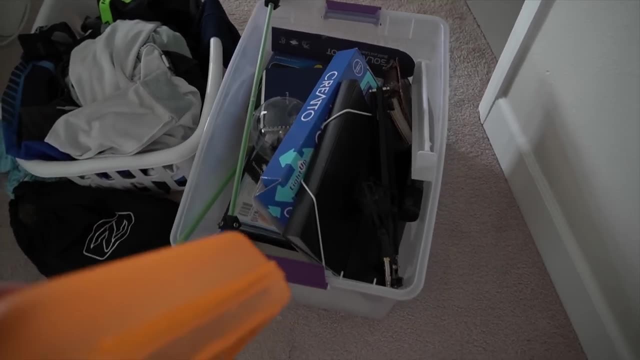 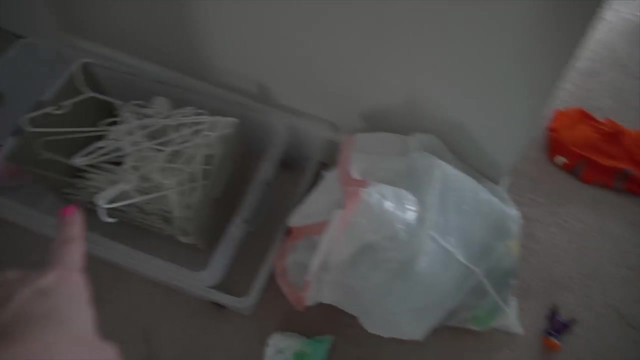 closet for a year, a year and a half. they've never touched. they are really good items, so like a whole art set building a robot, all the things. so I've got to think about the stuff like this because I just don't know that can be to dirty clothes, trash, a ton of hangers, bins with no tops, that's going to go. 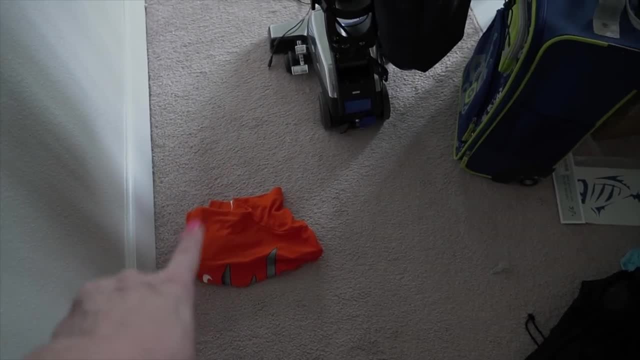 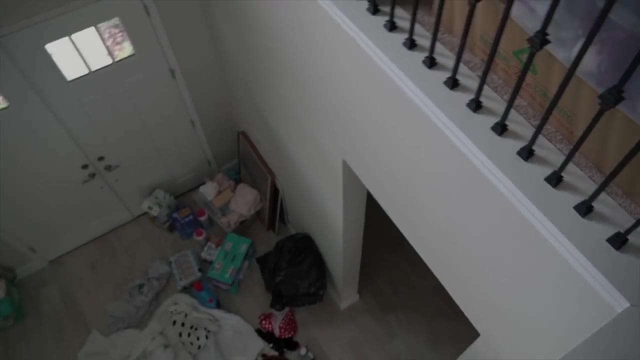 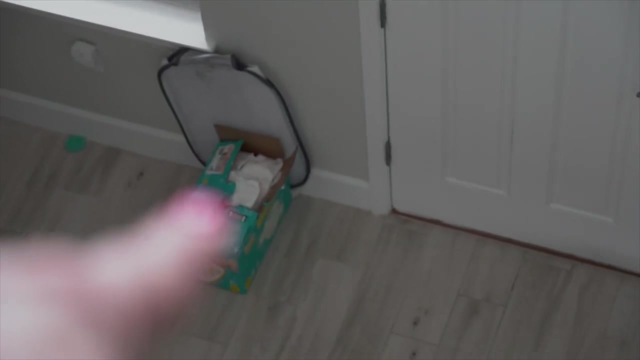 into the recycling. I gave all the clothes- the 8 to 10 size clothes medium- to a friend, but she has yet to come pick them up, so they're sitting right there and this is goodwill. and this is for a neighbor who's having a baby. this is: 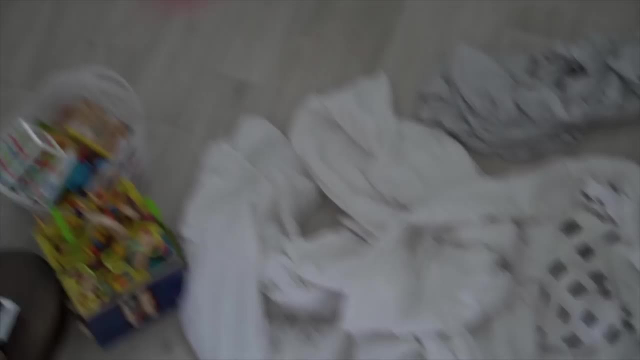 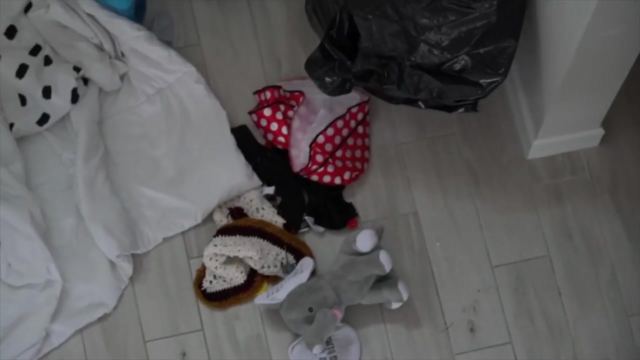 coming up here this stuff over here, cuz I'm gonna make a play area for Emma. this is the dirty clothes that I'm gonna wash now and this is my Sam's order and that's my Costco order, and then that stuff I need to find a home for over here we are. 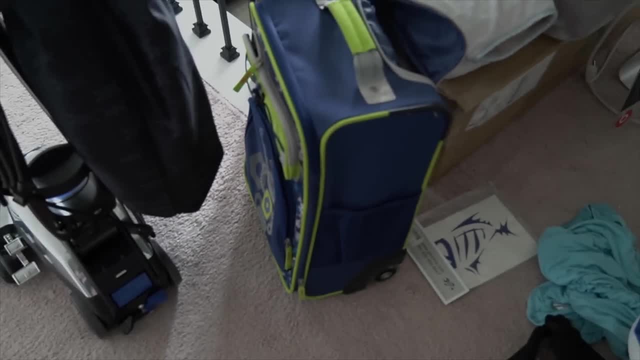 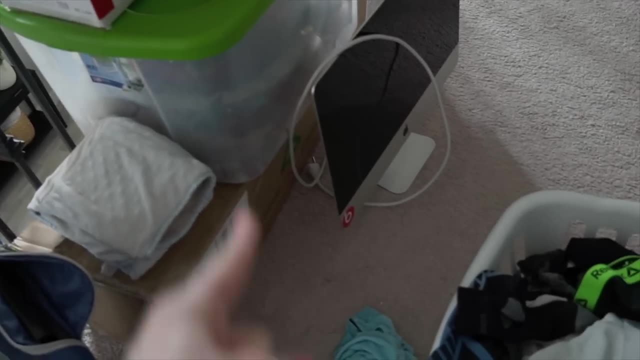 gonna get rid of this. I will donate it to somebody. I know they could use it. that's Josiah's blanket when he was a baby. I got to put it in his memory box. this is Christmas. yes, this is Christmas. my old Mac, I gotta figure something out. 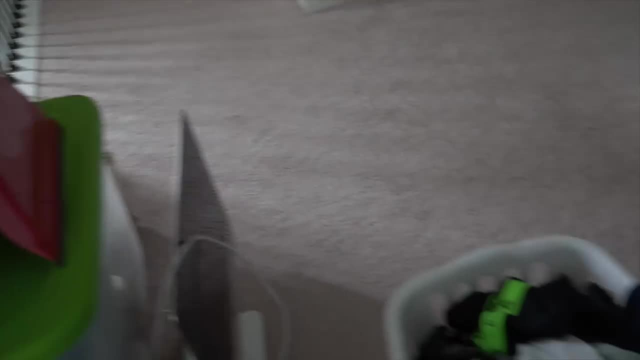 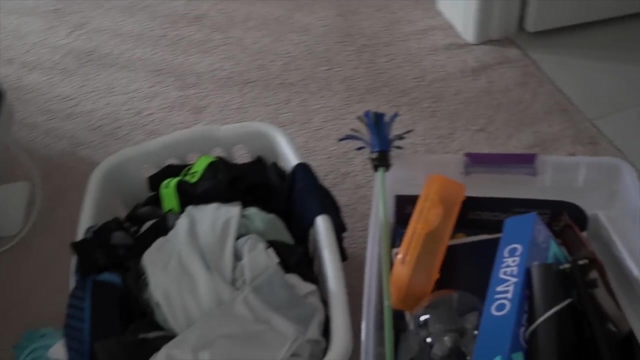 with that and that is terrifying. so here we are, bathroom still pretty much okay because I just got the clothes. so here we are, not too bad. I told you guys in my last video I haven't been feeling very well and I'm still battling cove it I. 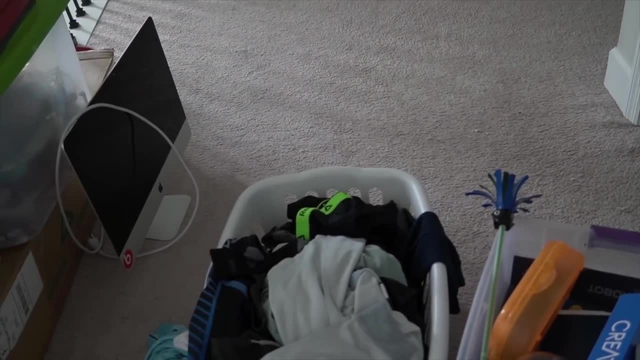 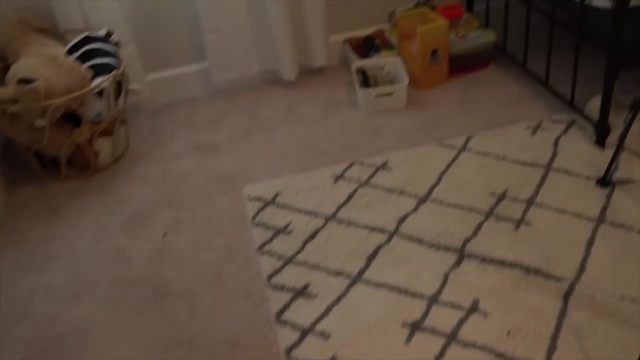 think I'm on day 10 or 11 now and it's it's kicking my butt. I'm not gonna lie to you, it's kicking my butt. I had to hold on. let me look at the camera. it took everything in me to get dressed. it's like everything in me to get. dressed. this morning I have been feeling like city viens. around. twice I started shooting at highest ground. you know what I heard. most of you said shoulder or something. so I've been loading up on ibuprofen and Tylenol, which I don't. 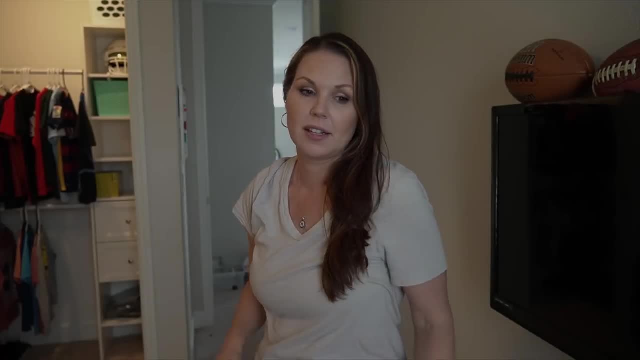 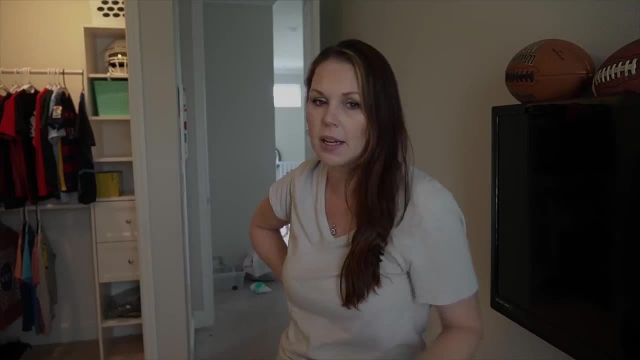 like doing, because I know how bad that is for your liver and your kidneys and your stomach and all that stuff. but like there ain't no nanny here, My husband ain't here, Ain't nobody here to help me And I don't like you gotta figure it out. 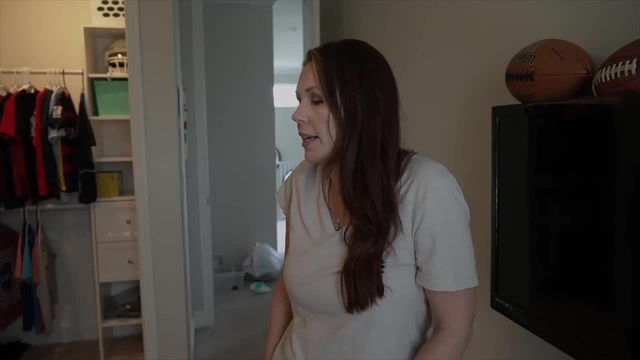 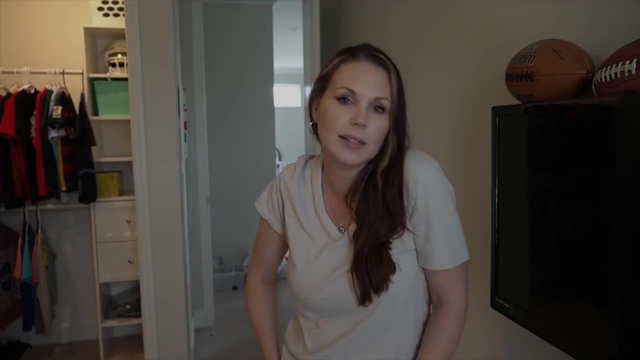 That's just what moms have to do, So I'm finally getting back at it. The previous clips were actually from over a week ago, So I'm getting back at it, but at least I'm doing it. I don't care about. 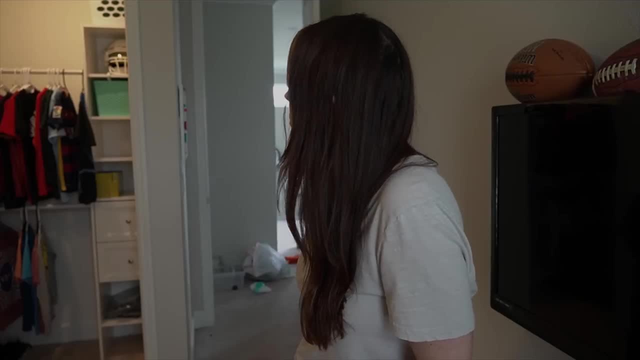 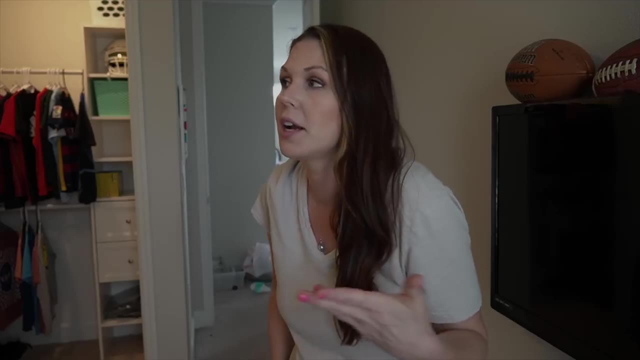 the time frame, and I would say the same for you. I did want to say- and I don't know if I'm gonna already say this in a voiceover or maybe saying it twice, so I'm sorry, but pay attention to the clothes that you're washing. and 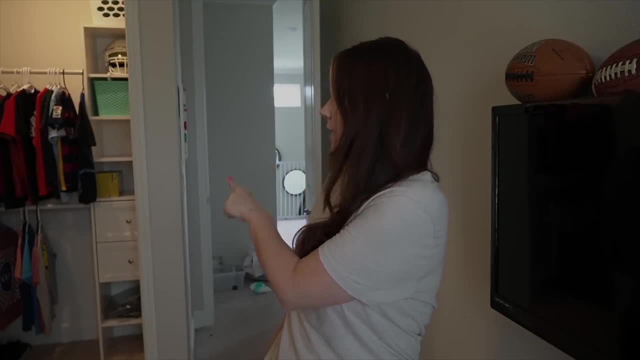 pay attention to the clothes that you're not washing, the ones that keep staying, that keep being hung up. Some items in there are for like they have, like Christmas programs and stuff like that. It's a black shirt and then another nice black shirt. 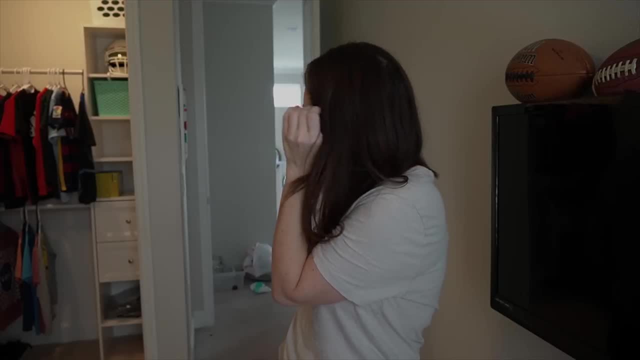 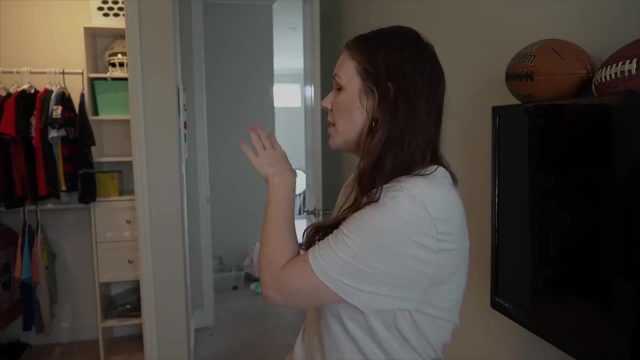 I'm gonna keep it. Then you got your hoodies. We don't wear them every day, But then the rest of the clothes. pay attention to that, Pay attention to what you're constantly seeing in the laundry and pay attention to the things that are always staying. 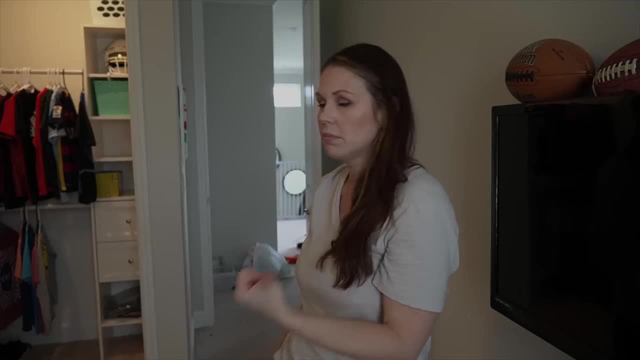 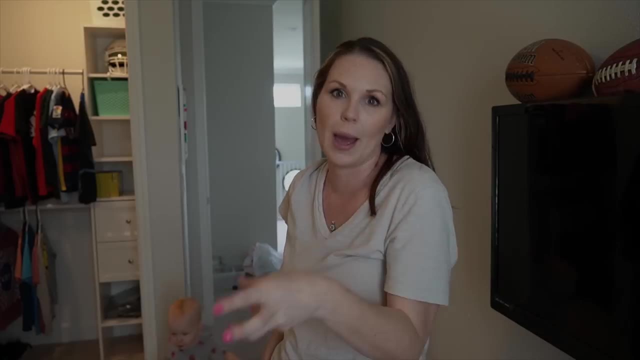 hung up because they're not being worn. The things that aren't being worn, go ahead and get rid of them because you know, unless it's something for, like a school program or something you know that's not what they're grabbing to If they're not. 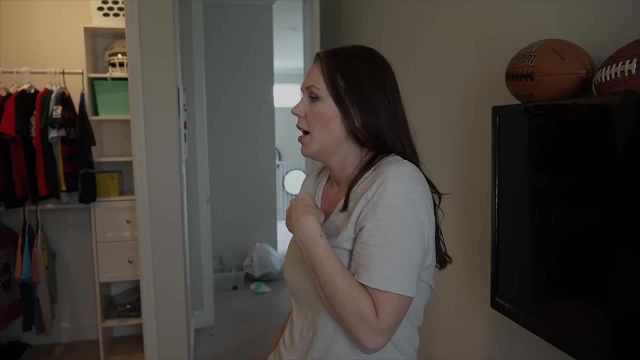 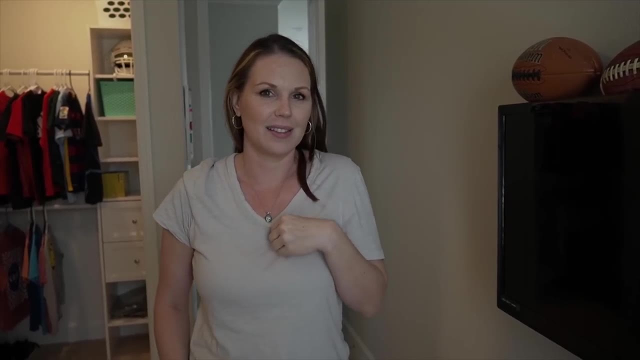 grabbing to it. they're not gonna wear it, and I'm learning that for myself. I had gotten rid of so many clothes and I figured out what I like. I like neutrals. I like things like this. Sorry, if the camera moves, That's Emma. 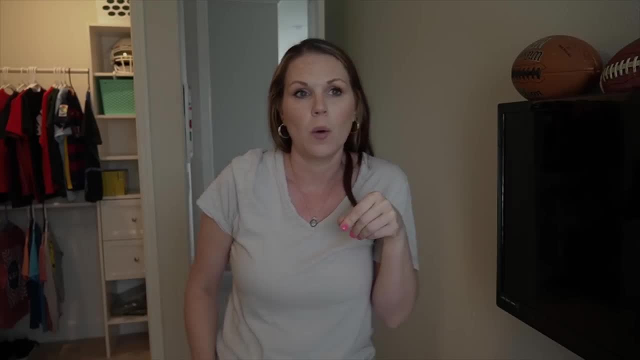 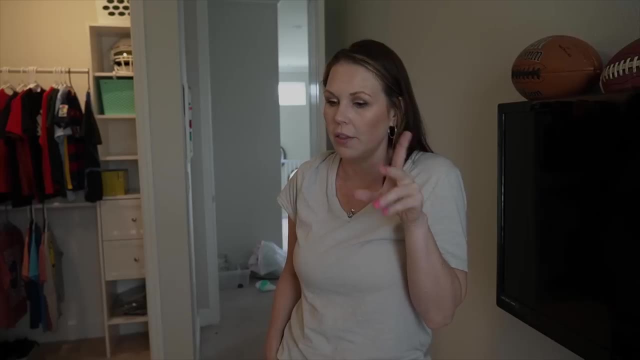 And when I would see things in the store, I would buy it. Well, the problem is is I've added a lot of things back to my closet that I don't even grab to, So another key tip is: stop bringing stuff into your. 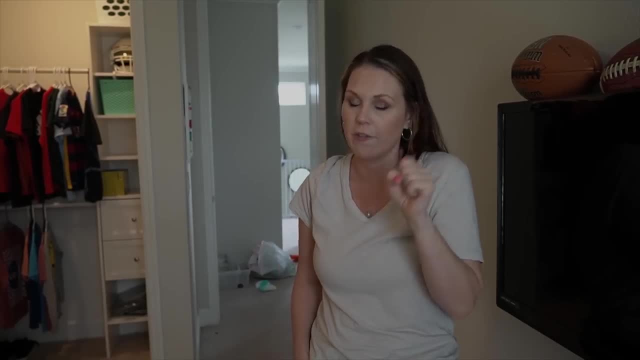 house. You can declutter all day long, every single day, but if you keep bringing stuff into your house, you're just gonna tire yourself out, and that's what I've learned about myself. I've tired myself out. So, yeah, this is good. 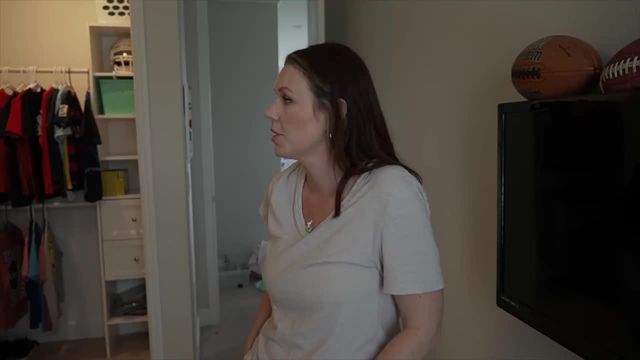 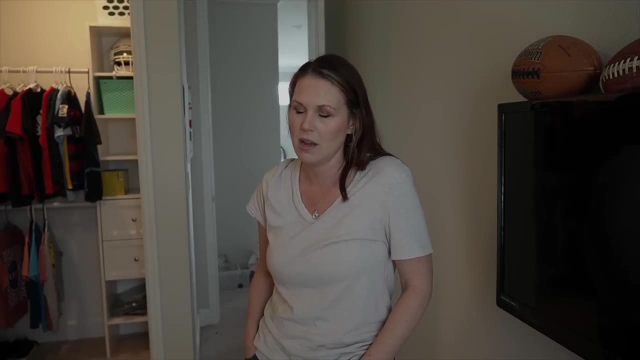 I'm doing good, though I haven't been bringing anything else in the house. So you know, I think when I'm in like a low mood, I end up often spending money that I really shouldn't be spending. I don't know why. 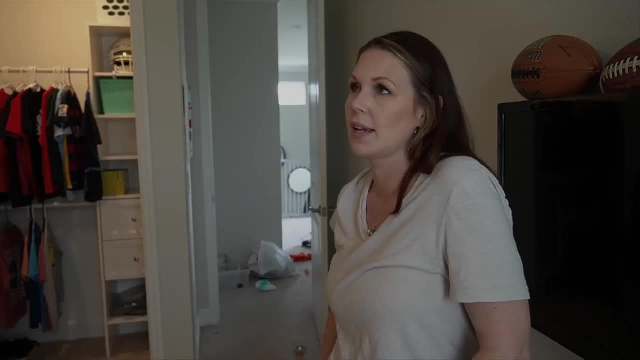 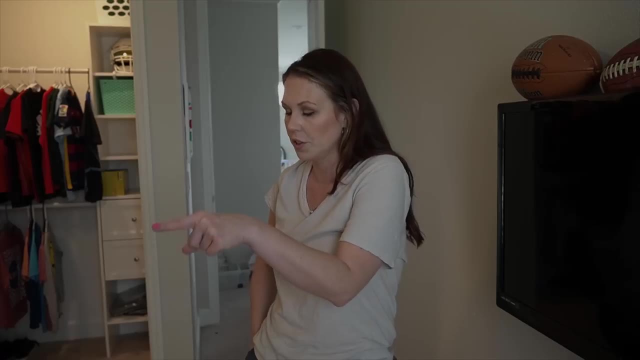 I actually do know why, but I won't get into the scientific information about that because I do know why. But yeah, feels good, looks good. I am now going to move this stuff onto their bed, pull the rug up and we're gonna vacuum with the. 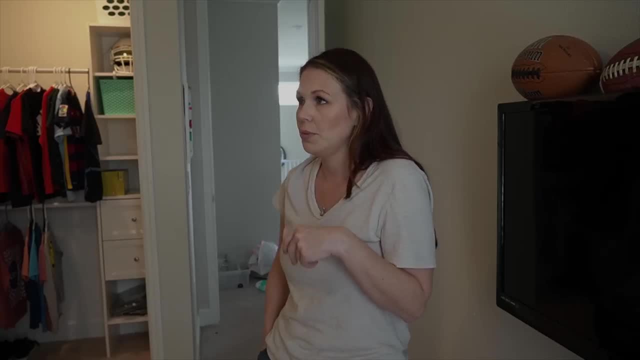 Kirby, because you know it's the big boy, It's the real deal, And this room needs to be dusted, so I actually will dust before that. Before I do that, though, I am gonna have Josiah look at all of his little figurines. 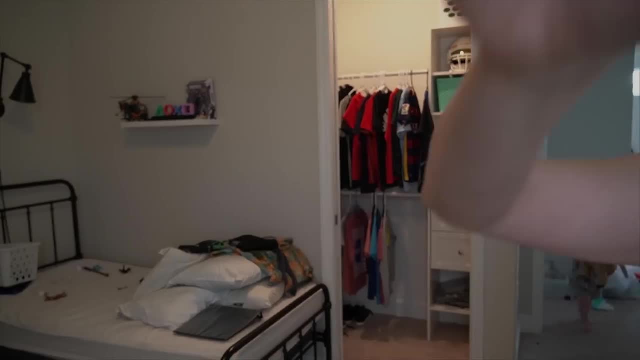 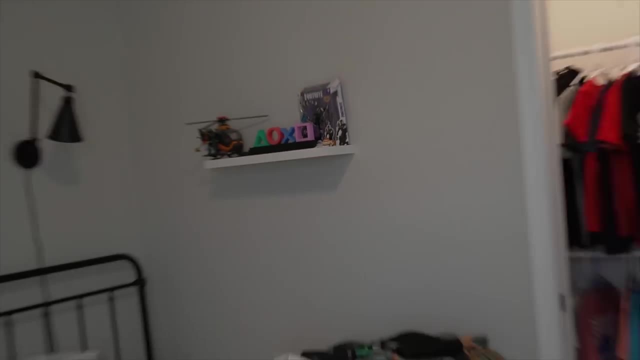 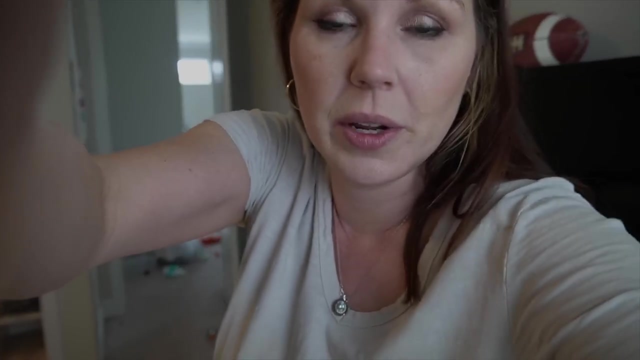 Josiah likes to collect things, So he's got a ton of figurines- Fortnite figurines- that he needs to go through. You see, He needs to go through all those. I was trying to get Emma. There's Emma, So we need. 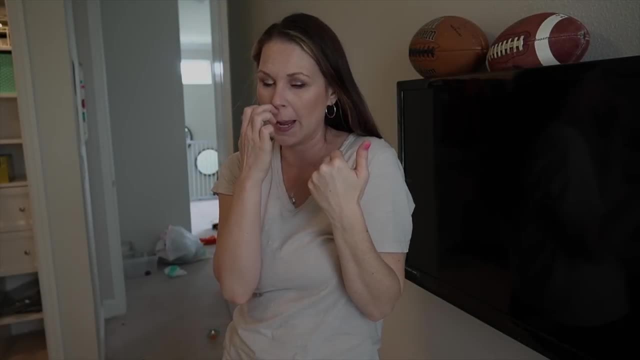 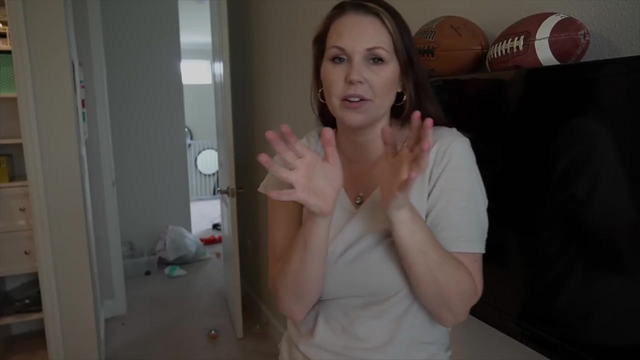 to go through some of that stuff because they're stuffy a lot and I- yes, there's a lot of illness going around- But I have and I think it's the dust. I think it's the dust, the dander in the air, and this needs to be. 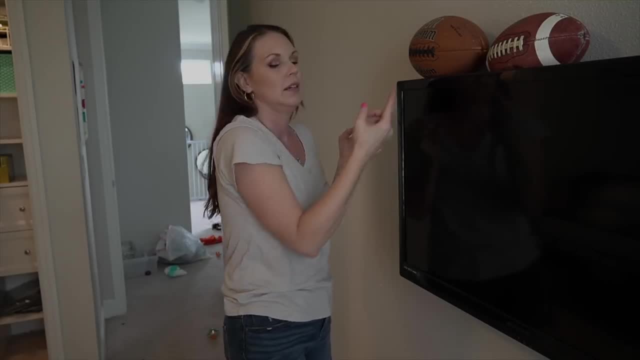 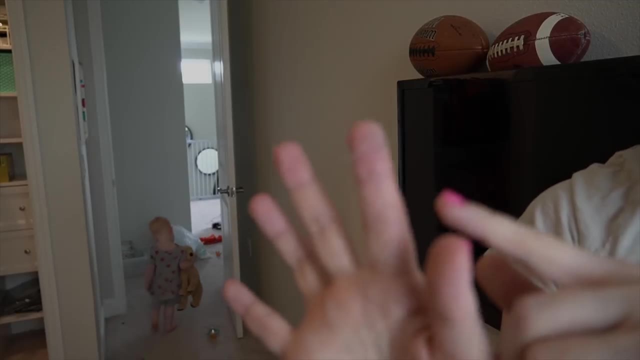 taken care of while I'm standing here. Let's just take a little look at it. Yeah, Let me see if I can like focus. Sorry, I don't know if I can, But anyway it's a lot of dust. 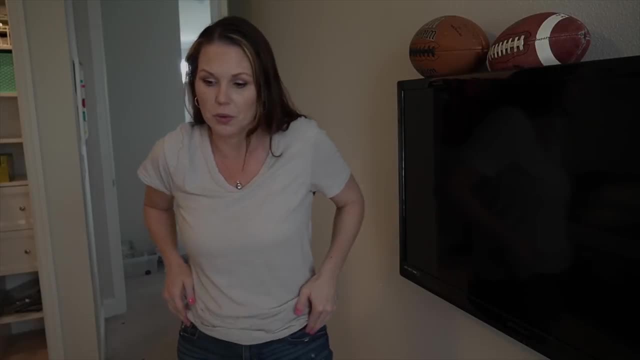 So I need to clean that. So, yeah, Alright, We're getting, we're doing good, We made a lot of progress. That big old bag of clothes, that was good. Um, I guess my friend's going to take it all. I can't pick it up. 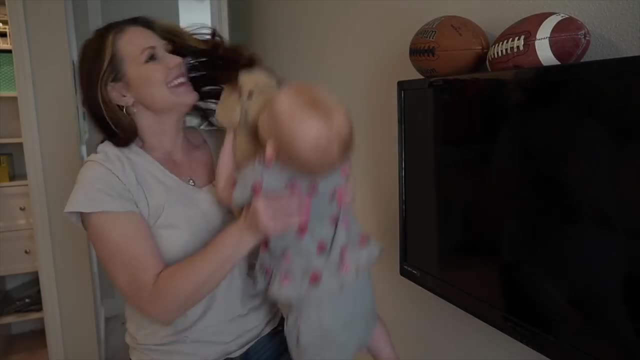 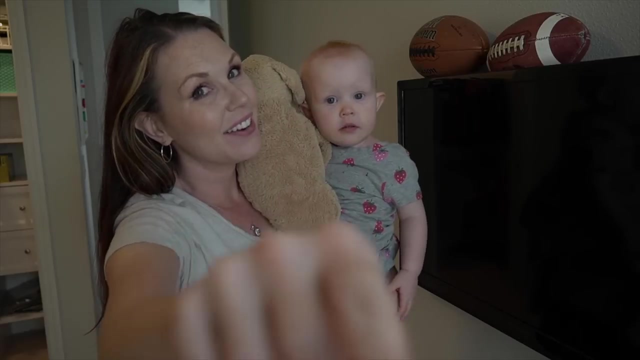 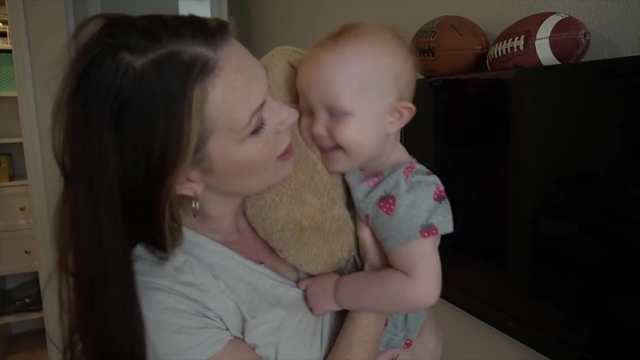 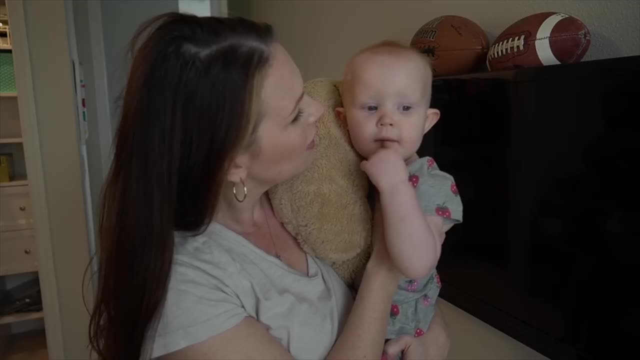 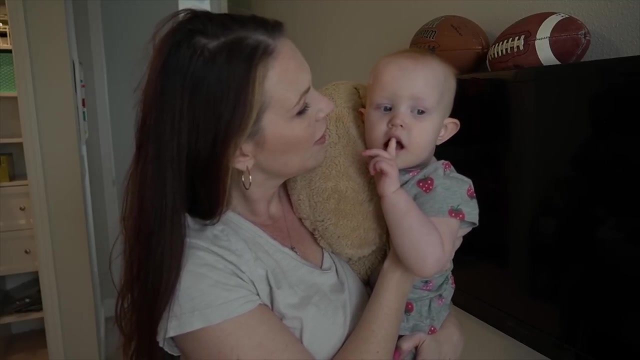 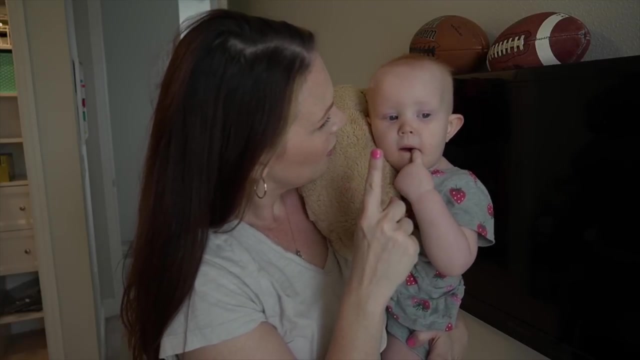 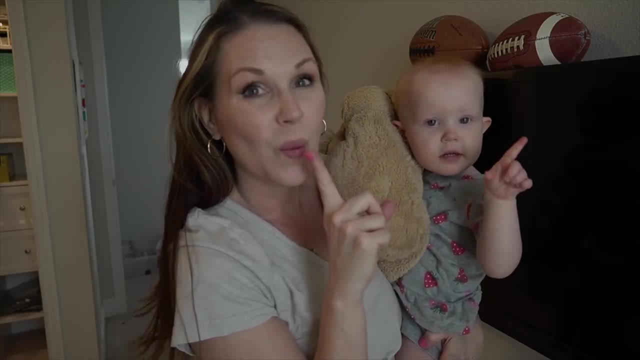 Emma, Emma. Hi, She says: my name is Emma. How old are you? How old are you, Emma, Emma? How old is Emma? How old is Emma? Is Emma one? Do your finger One One, Emma one. 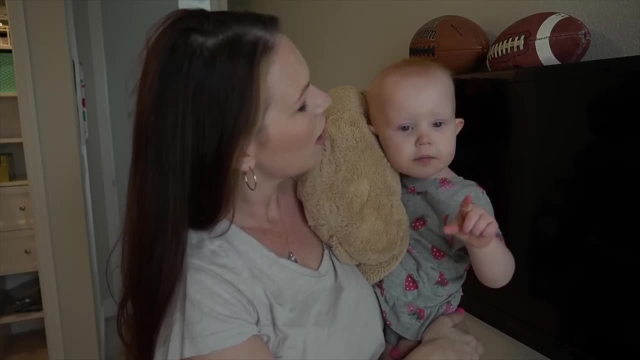 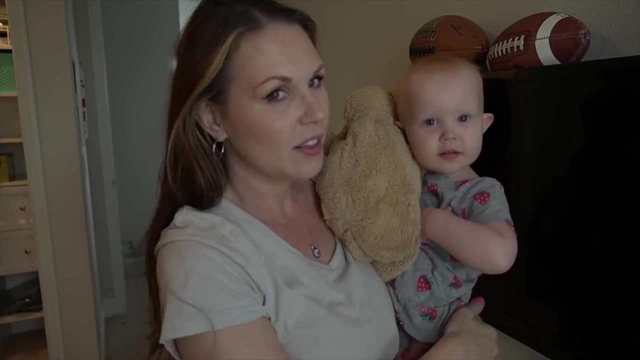 One, Emma. Emma is one. Say Emma is one. Emma wants to ride. Yeah, What's my name, Mommy, And who are they? Say those are our friends. Say friends. Say those are our friends. Two friends: 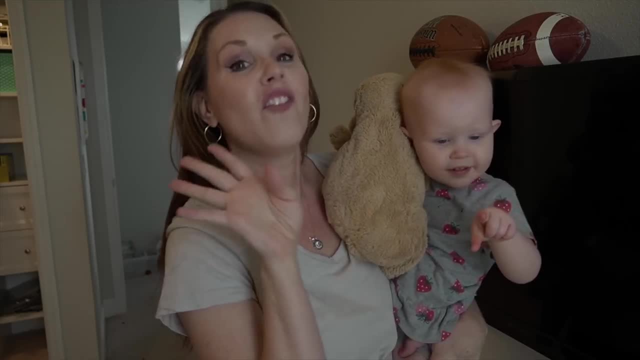 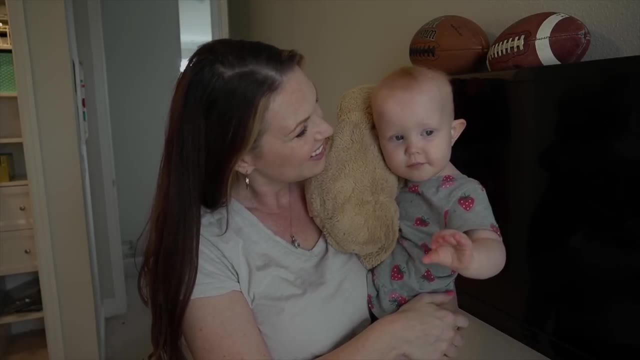 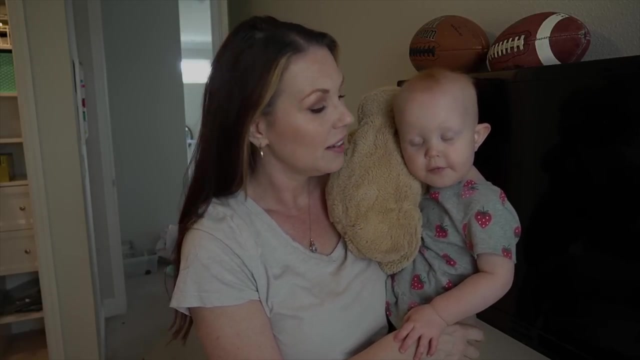 Two friends, Four friends, Four friends, Five friends, Five friends, Our friends, Our friends. Can you say: love you, Love you friends, Love you friends. Okay, That's too cute. We're going to stop right there and get back to cleaning. 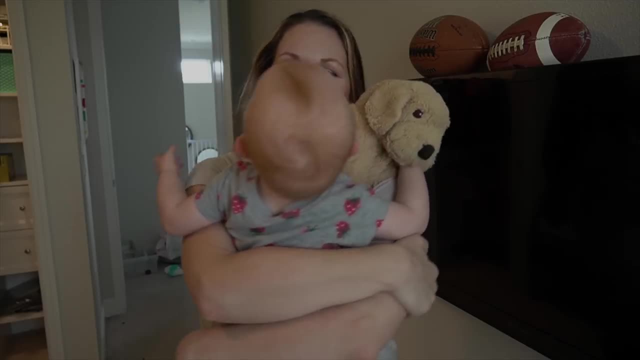 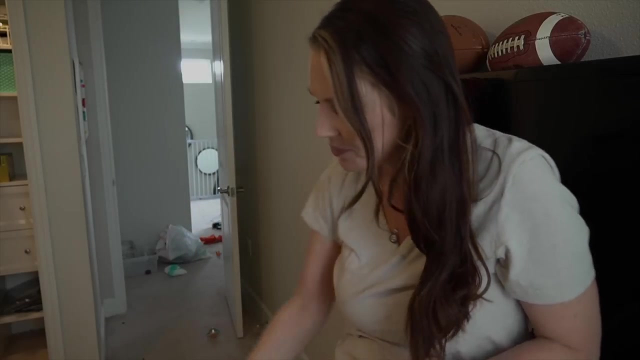 I love you so much, Mommy, I love you. Okay, All right, Back to it. Back to it, Mama, Huh, What is he Speaking of? toys we need to get rid of. He's so cute, though, but he collects dust. 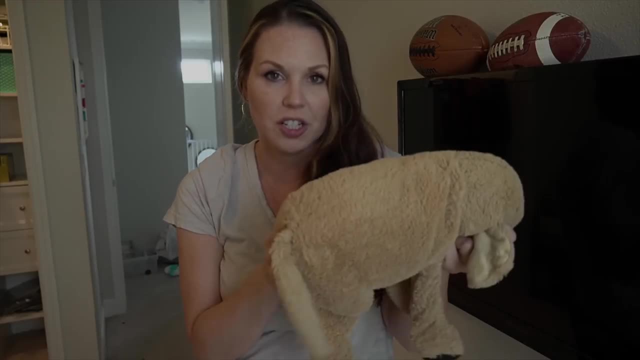 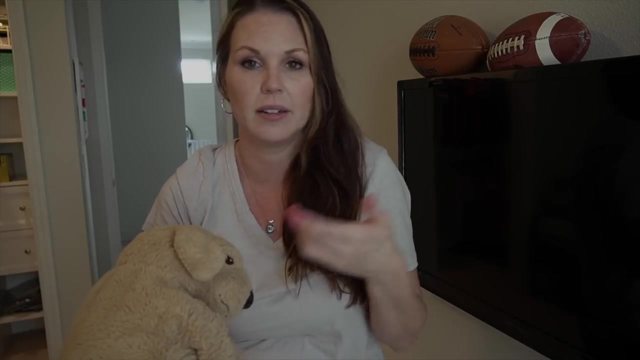 Oh, I did want to say this. I don't know if you know You can wash your stuffed animals. You might know that. but if you want to kill dust mites- and even I'm just gonna throw this out there- if you ever want to know lice or anything like that- 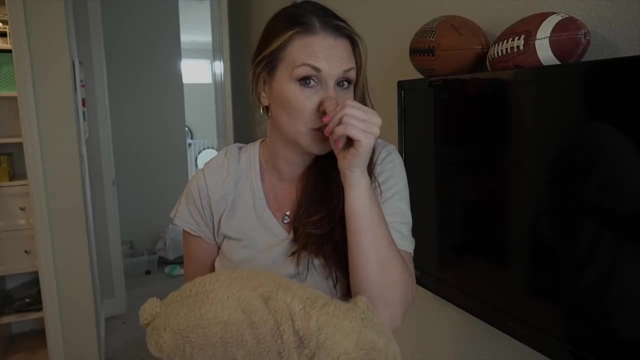 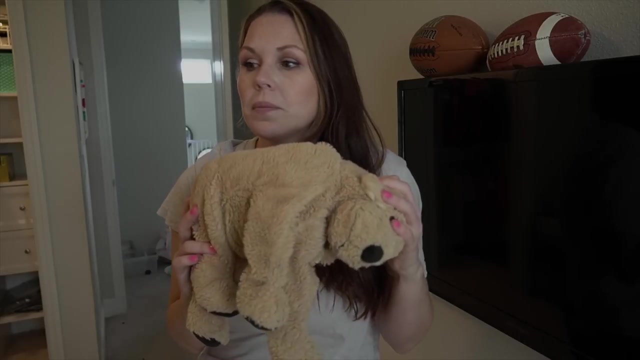 bacteria in your clothes, just throw them in the dryer. you don't actually have to put them through a whole wash. if it will withstand a wash, do it, but if it won't- because some toys won't, they'll get all yucky inside. um, just a dryer on the highest heat. I didn't know that one time my kids 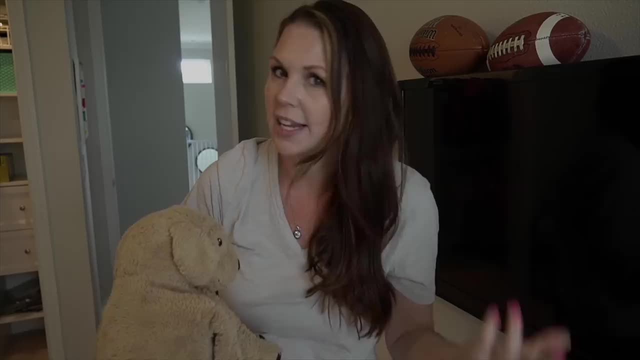 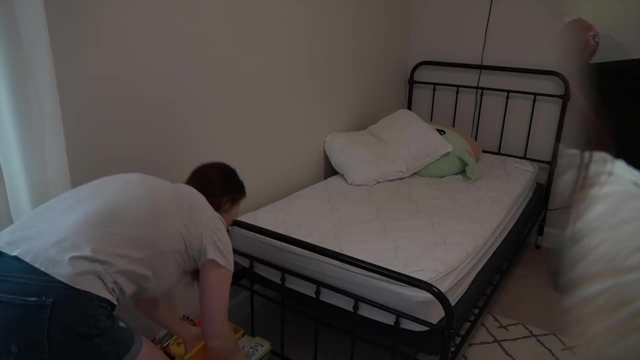 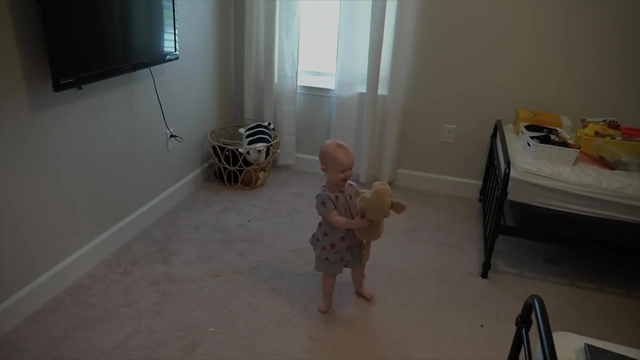 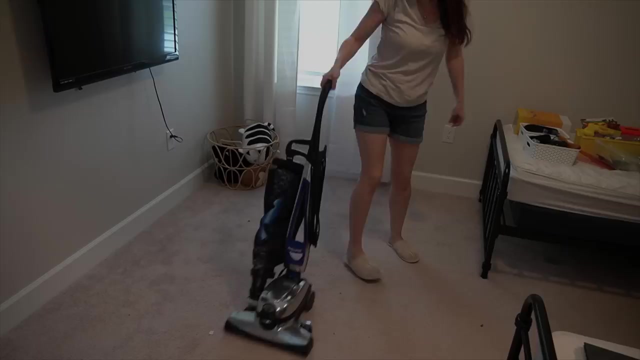 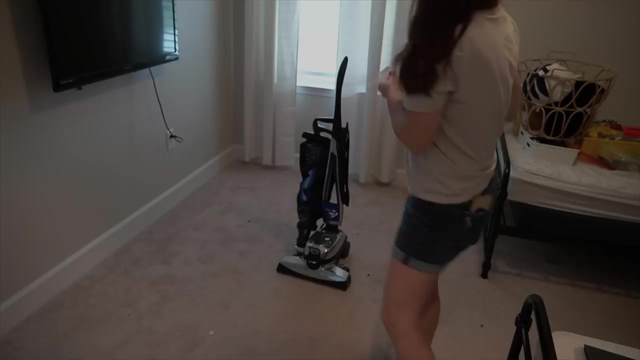 had lice and I was washing everything in the house and then a professional lice person said you can just dry it and she's absolutely right. so the more you know right, the more you know. I can't hear myself now. every day since I woke up I can finally. 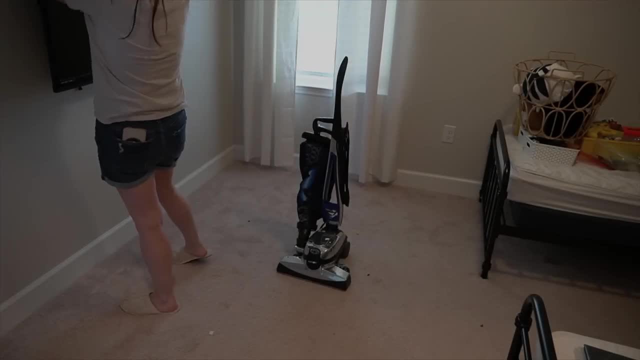 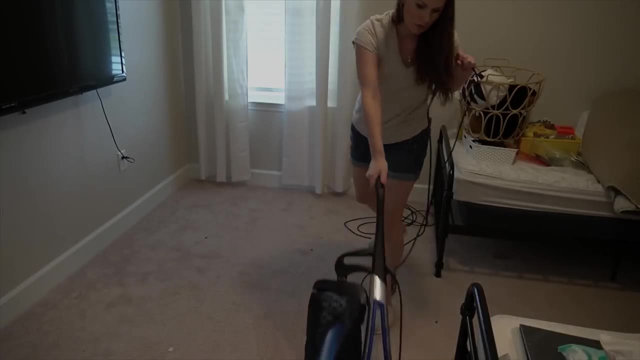 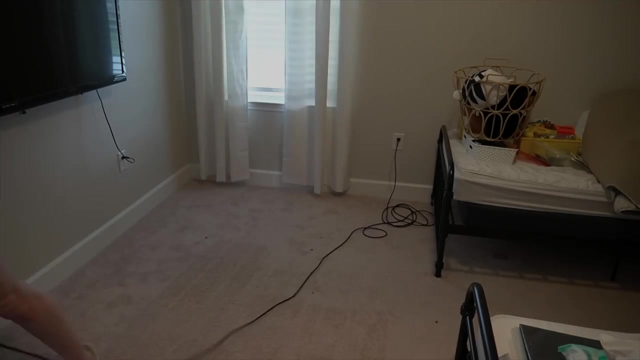 see. so you guys already know on this channel we improvise where we have to. so I used a baby wipe and wiped down all of the surfaces really quick, which worked beautifully, let me just add. and then I'm going to vacuum. uh, Emma is right outside the door now. we have gates, we have stairs. 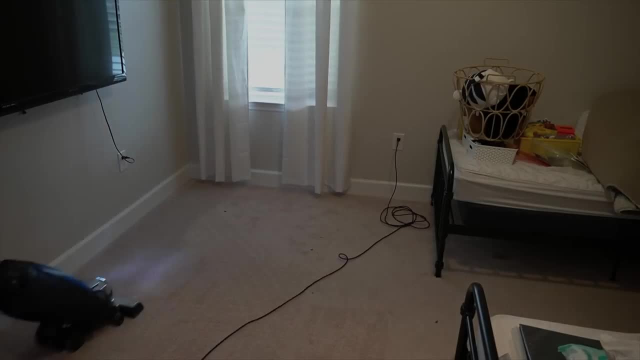 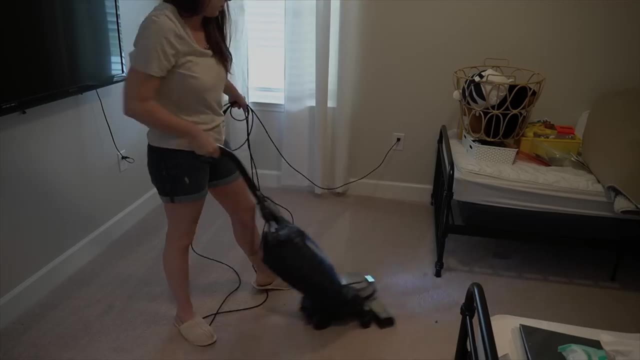 we have gates at the top and gates at the bottom, so she's completely secure and good to go, and I'm going to knock this out before the boys come home and then I will have them look through some of these items and I'll see you guys in the next video. 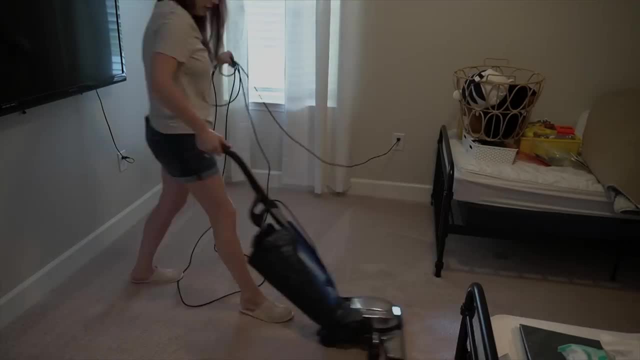 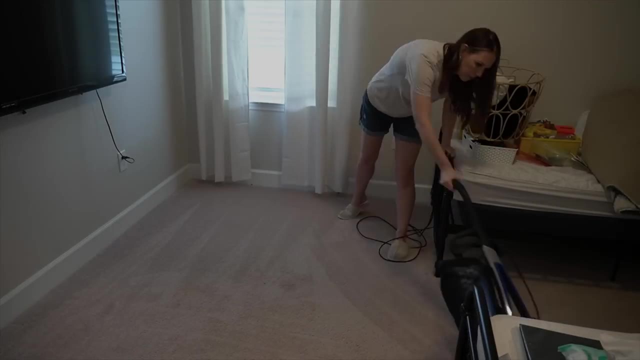 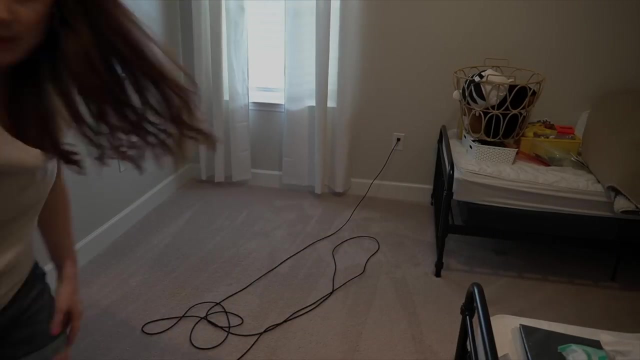 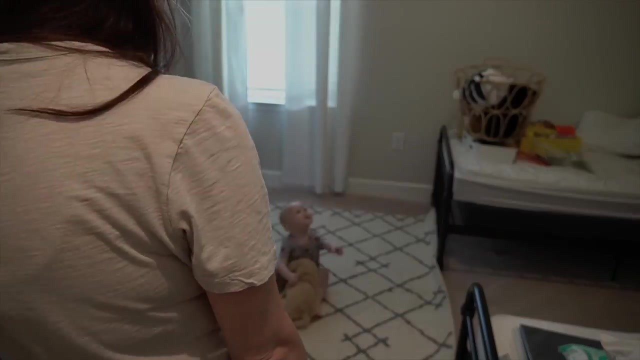 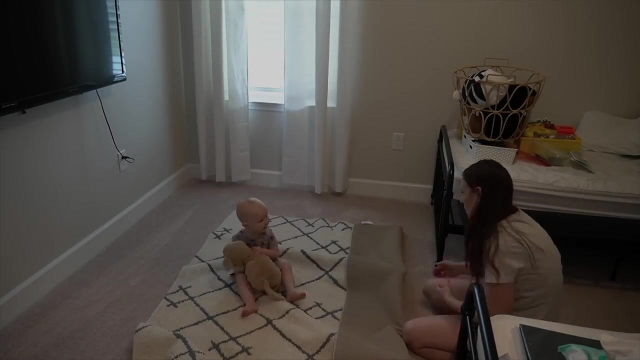 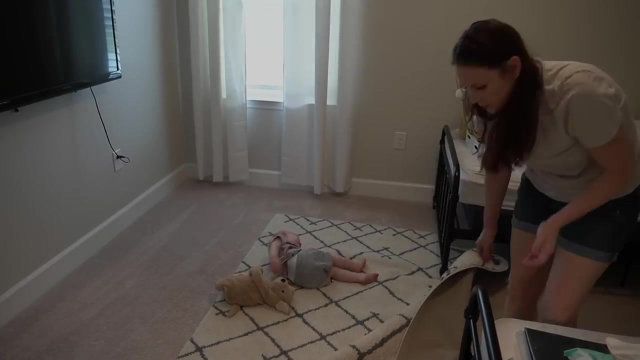 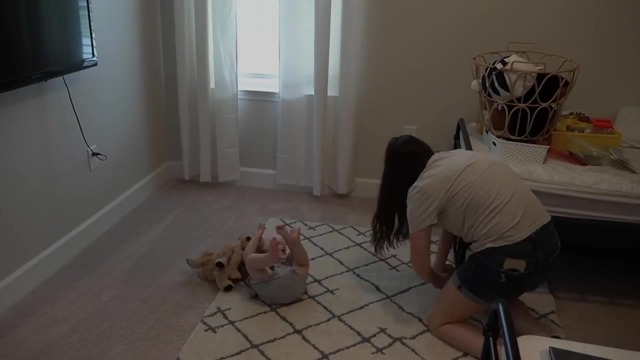 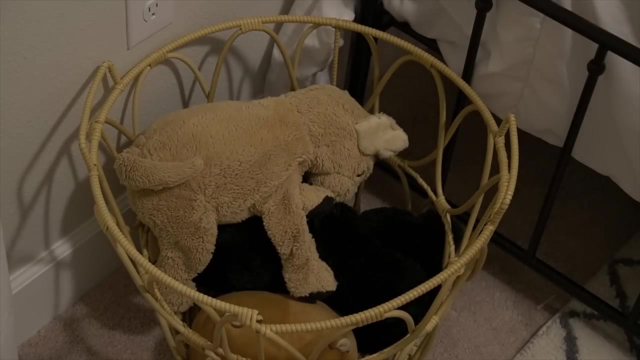 but I love this vacuum because I know that it's doing a deep down clean, but it's just so incredibly heavy, but it's worth it because they are laying oh so quiet. nói líон, you, you, you, you, what? yeah? yeah, this is size, so we're going to keep that yeah. 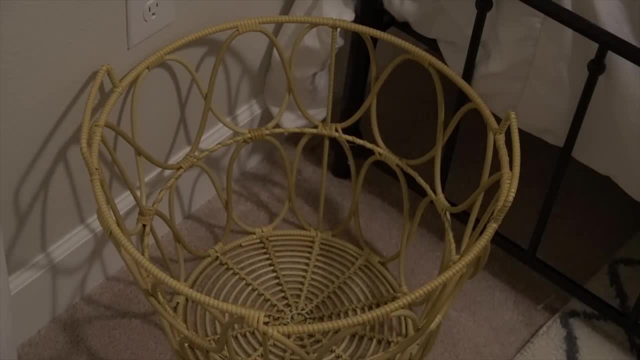 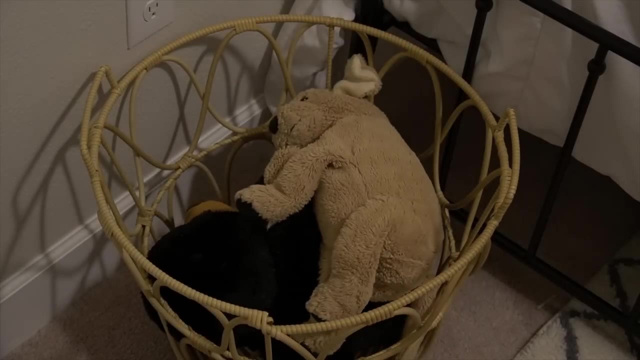 this one. so throw in what you want. throw it in it. you don't? you keep them all. I'm just asking, just but just, you should make a choice. what are you gonna hold on to? what are you not? um dog, yes, those are, that's for sure. memories, okay, memories. 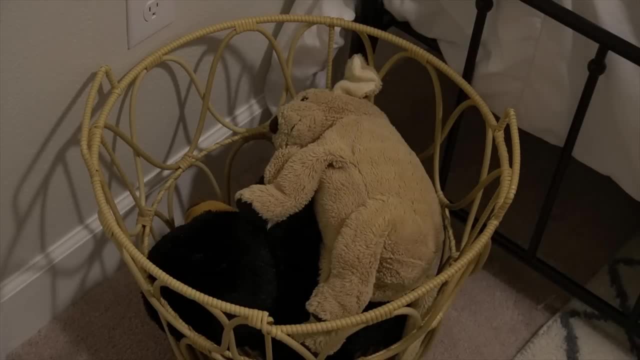 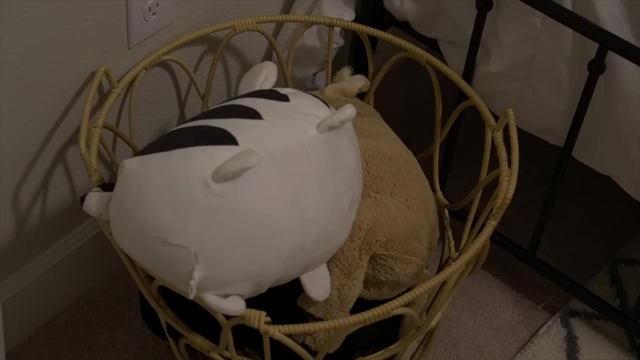 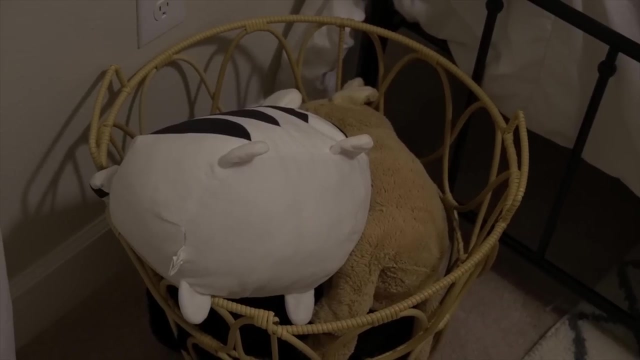 like a lens, of course. okay, keeping that. you're ready to let him go, it's okay yourself. well, you do have to stop. okay, you do have your one squash mellow, won't we get that to Emma? yeah, here we go. okay, good job, all right, okay, go take. 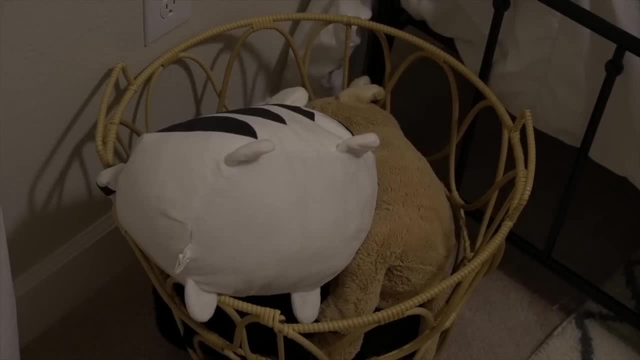 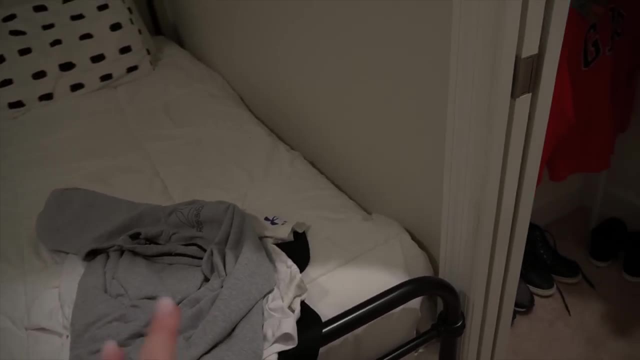 this and put it in the media room. love, okay, and then go get that, play it. we have homework to do, okay. so here is their closet. Noah has some clothes right here that we have to put away. I need to get them some more hangers out of my. 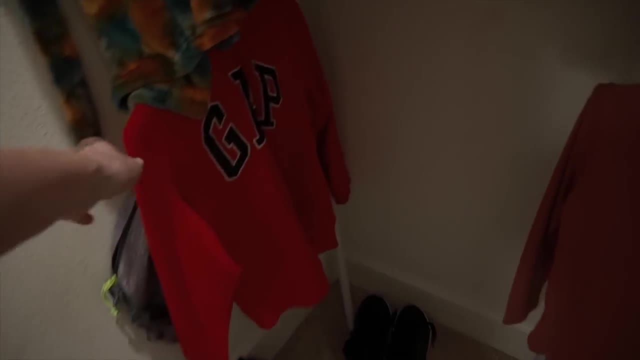 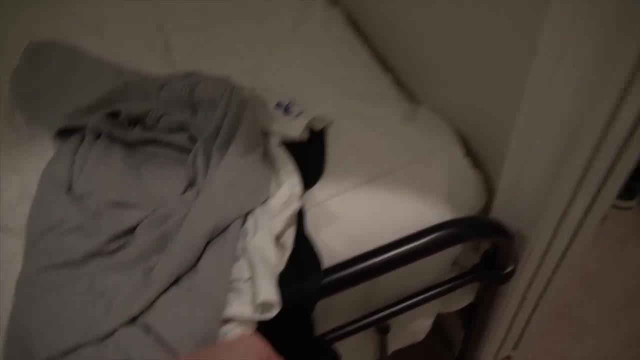 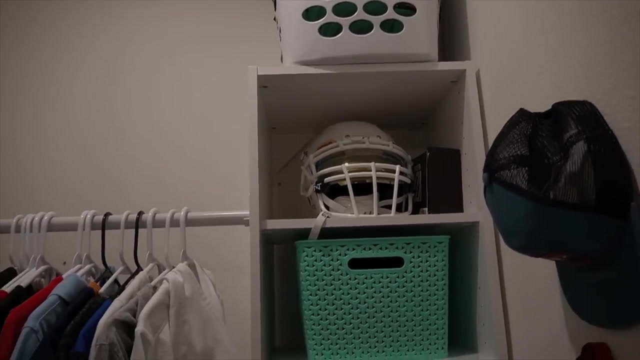 room, but this is what we're left with right here- not bad, plus these four items right here. here's your Josiah's clothes- much better up there. I've got clothes. I think I've already talked to you about all of those. I won't worry about it, I've got. 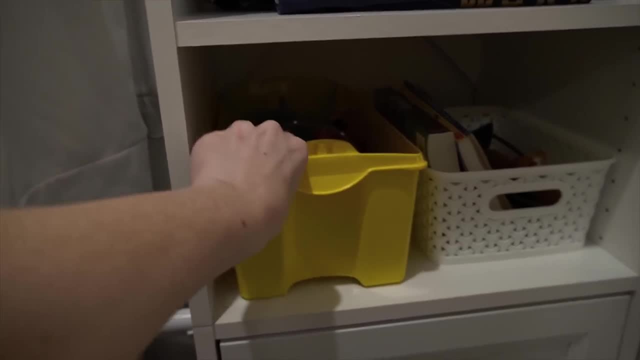 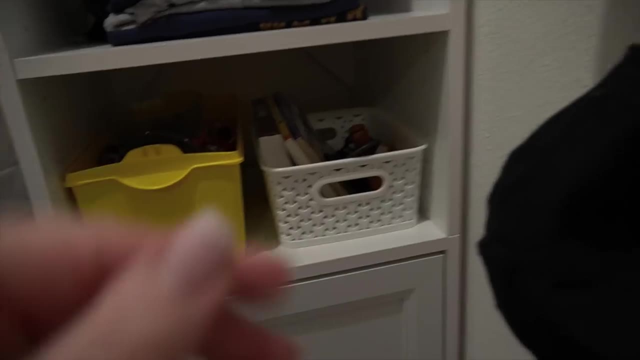 their school shirts, the Legos that Noah felt like we're really important and special, a couple of books and some miscellaneous items that we got at Georgia that they wanted to keep, and then I just used the tax to hang up their hats. I'm gonna use something to get something better. 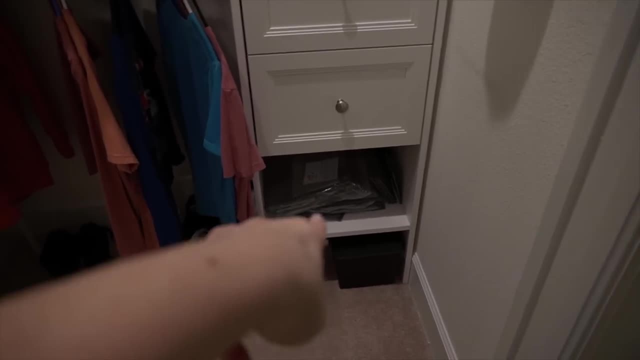 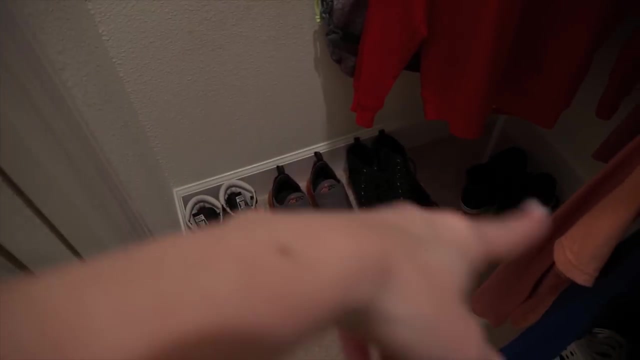 because they are falling down. I got a couple organizers right there that I'm probably just going to resell because I never got around to using them, and then they're shoes, play shoes, and I think I'm going to try to get him to get rid of. 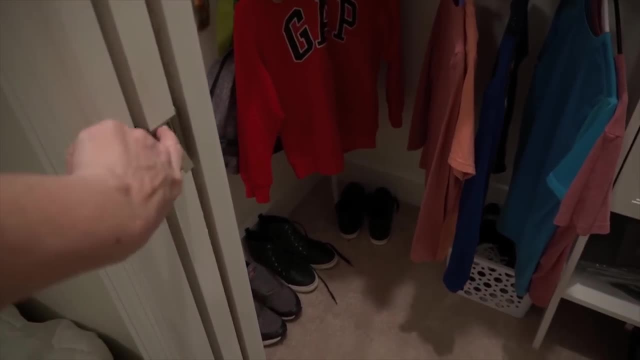 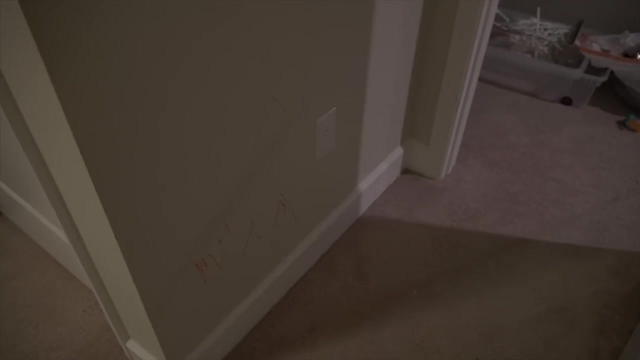 that was because the laces are out, but in my opinion, not too shy, okay. so here's. okay, I had a little filled day. here is their bedroom. you saw, Noah, the? here is their bedroom. he's sitting down near the keys in the kitchen. Mrs, because we're in here, I need to go in and get a 20 bar이�降여. 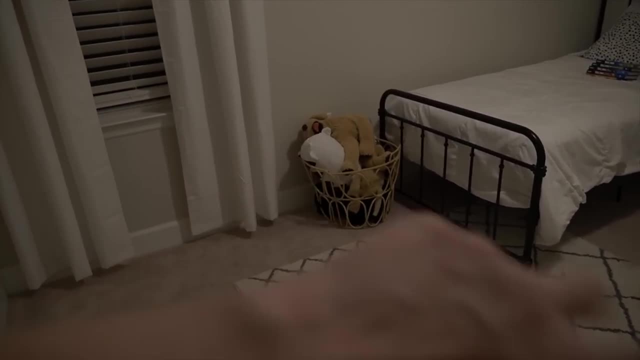 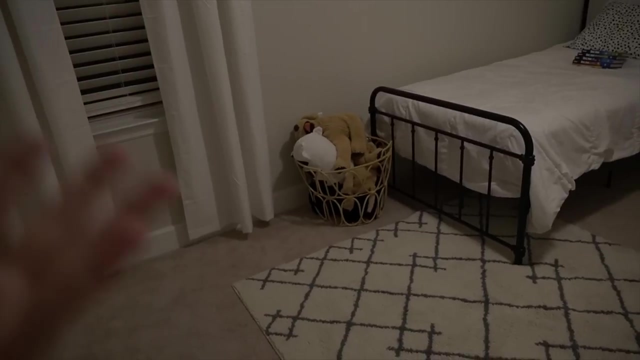 you saw, Noah went through his basket. He pulled one item out. I do not force them or push them to do more than they're comfortable with. I do encourage, like: okay, are you sure you're like? you know he wanted to keep it all And I said, well, or you know you're not able to play with. 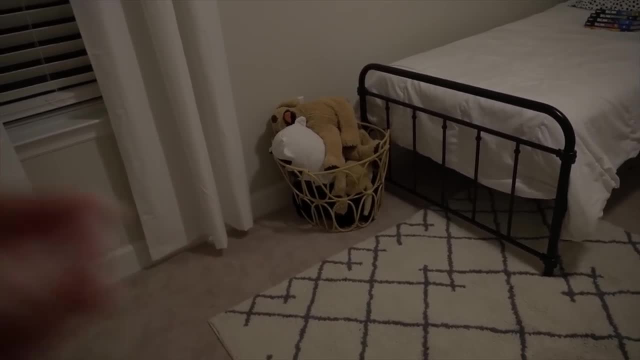 everything Let's. you know, I kind of try to do it like that. I make them think: and you didn't see his face because he just got out of the bath and he's not dressed. But he was like I don't. 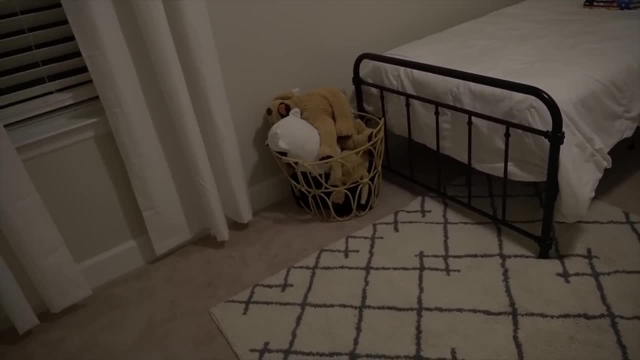 know It's so soft, I want to keep it And I'm like, yeah, but you know we could give it to Emma And that's a good transition for him. I think for kids, depending on your child, my kids, 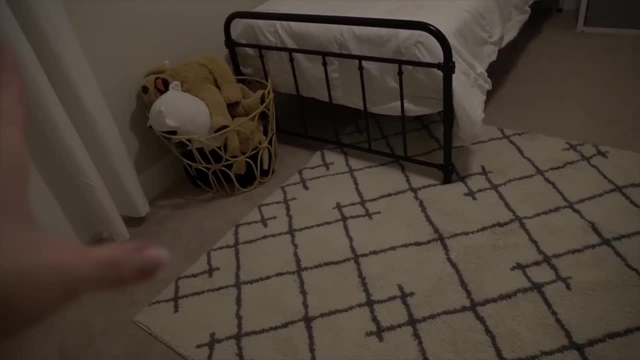 may need a little buffer every once in a while. Some kids like Liam, he'll be like throw it away. I don't care, Noah needs a buffer. Noah is like: oh so, let me just get it out of the room And 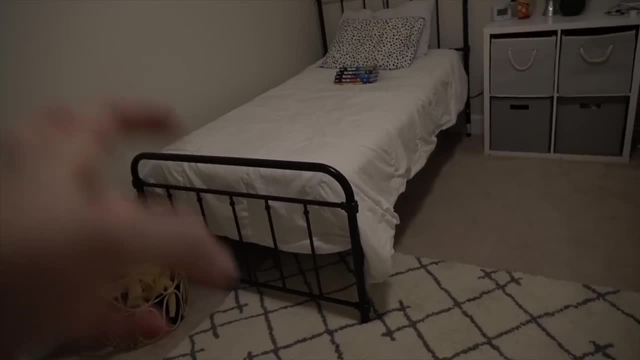 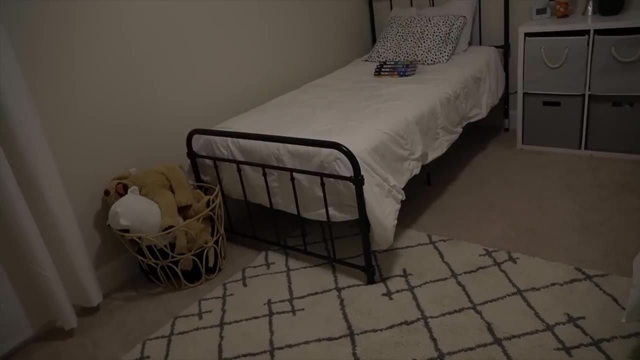 once I get it out of the room, let me put it downstairs for Emma. Once I get it downstairs for him, let me get it into the garage. And that is what helps him And it's just kind of breaking those ties a little bit. I also want him to know that mom's not just going to come in here and 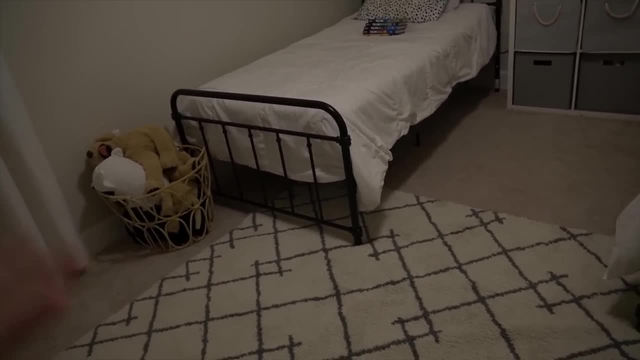 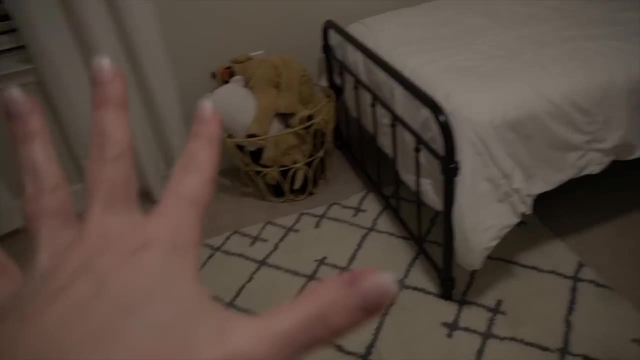 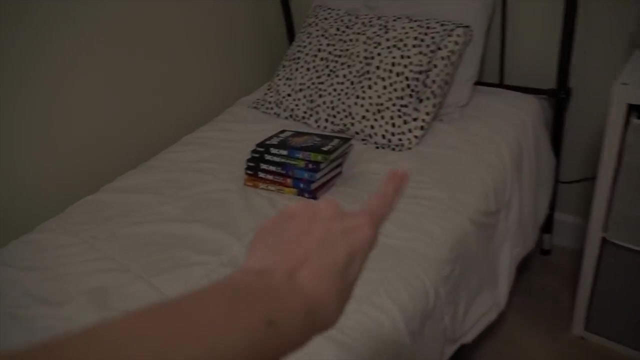 take all his stuff away. That's really, really important, because that can be really traumatic for kids. So you want to be sensitive but yet still proactive. The beds are completely clean underneath, except for over here. we do have their beddy bed in the bag, whatever it's called. 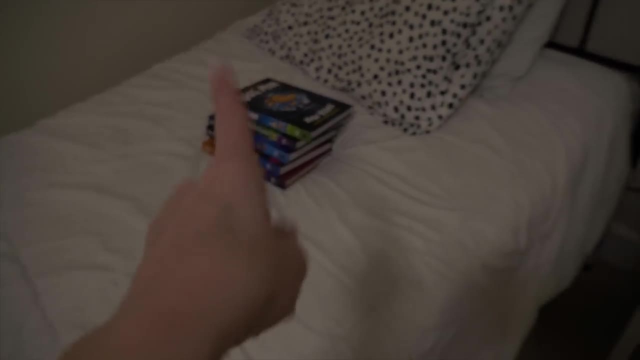 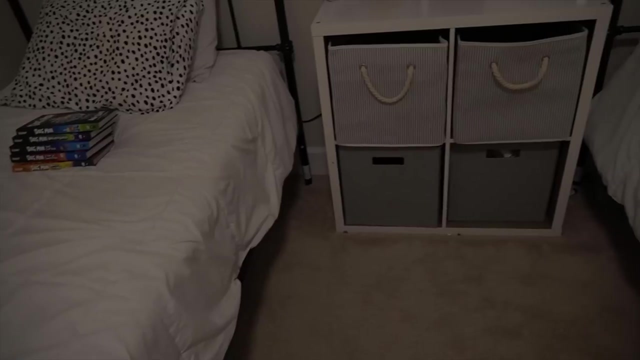 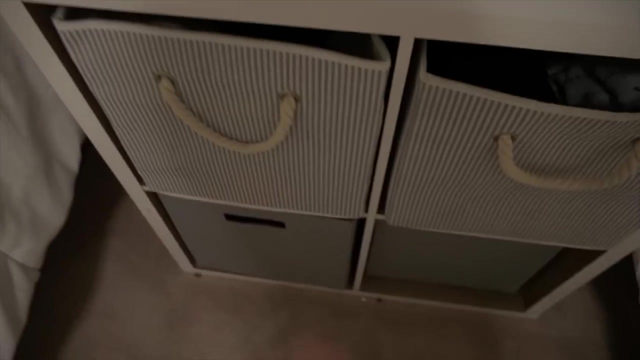 the zipper bed. I am going to go put those in there. I'm going to sell them. They read all of those books. No need to keep books that you've already read unless you plan to read them again. Organize all of their bins um all of their workout shorts and socks and underwear. Uh. 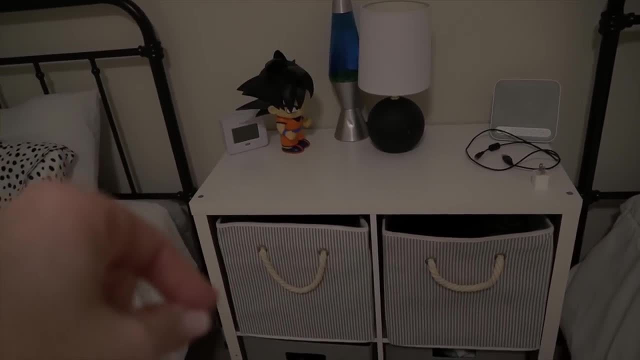 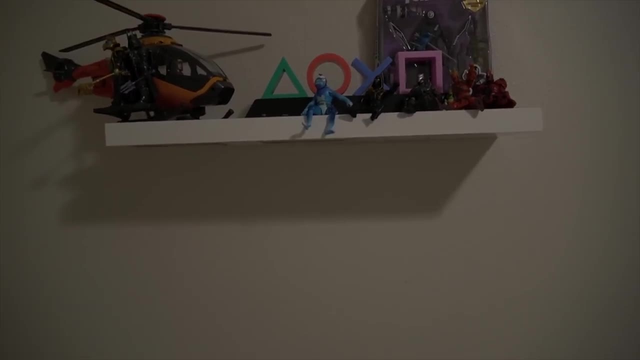 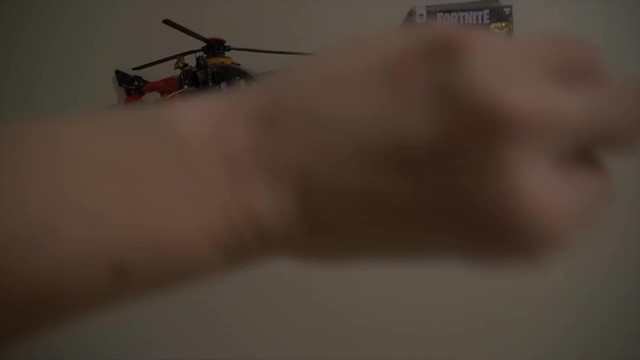 I'm going to probably get rid of that lava lamp. It doesn't work, Um, and I have yet to cut those things off. I had asked Josiah about his little figurines. He wants to keep them and that's okay because they're all right here. So I would consider this like contained clutter. I don't. 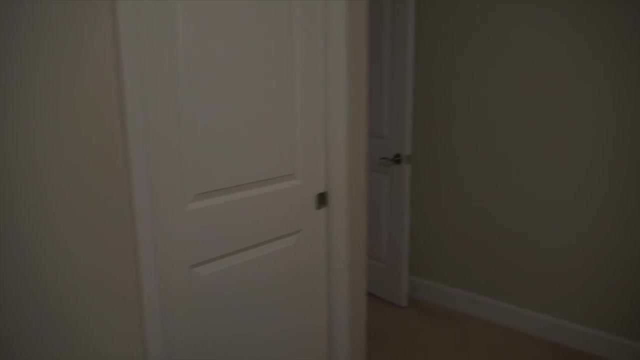 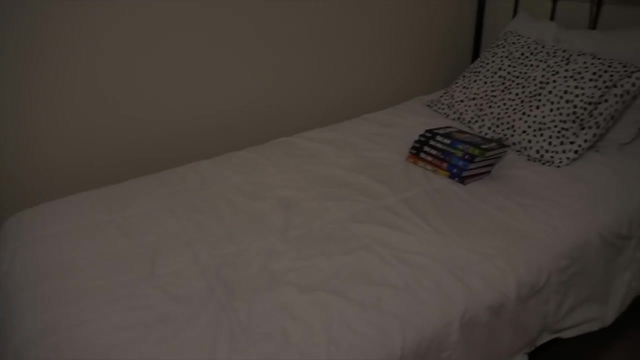 love it up here, but look at this room. It's pretty open and bare. So if he's going to have one shelf that has memorabilia or something special on here that he wants, I'm going to let him have it. I'm not going to fight with him. I'm not going to fuss. 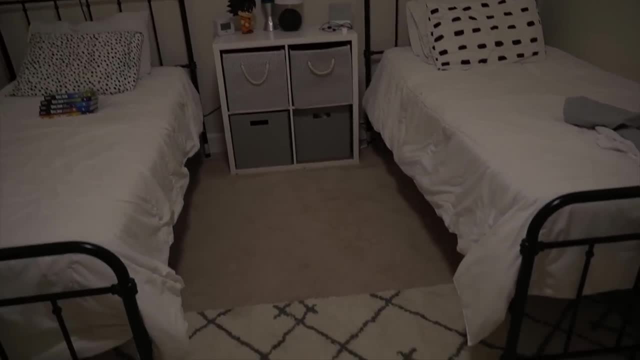 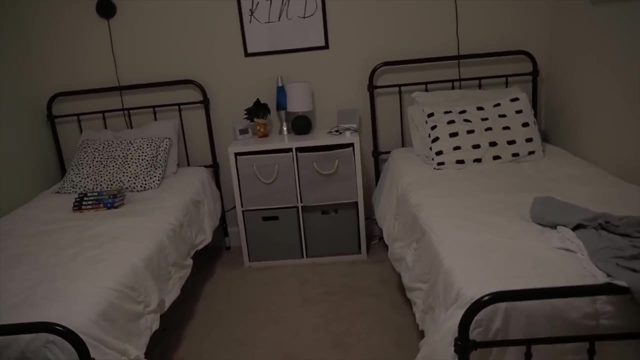 over it. Um, eventually I may ask him if he wants to put it in a special box or donate them or even sell them, And then I'll let him have the money for them. but that's on his own time, And I try. 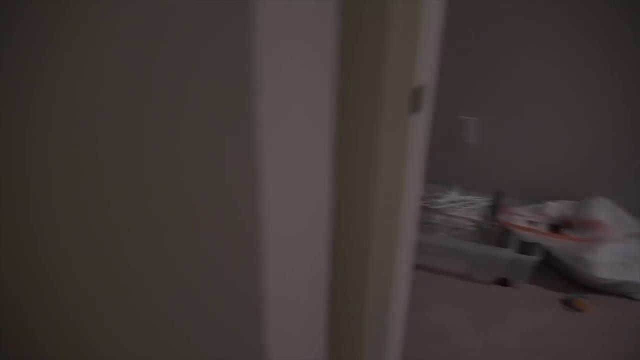 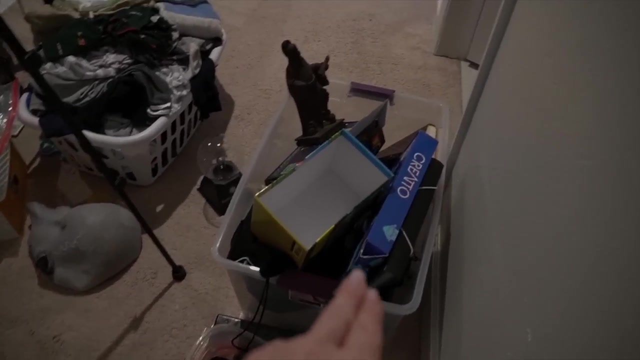 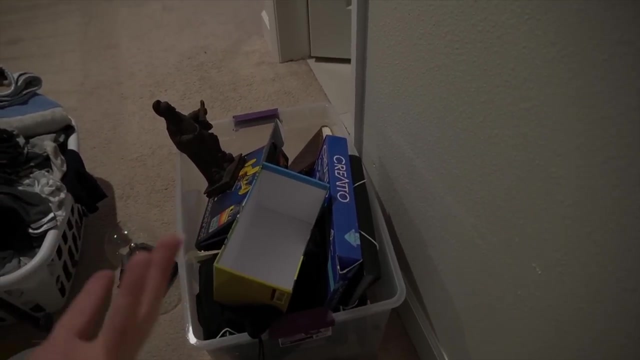 to do that. So now let me show you out here. Oh my gosh, So this is how it always goes. This is all the stuff from my room. I was going to have them go through it, but I decided not to because they haven't touched it in over two years. You don't need it And it's literally just stuff. 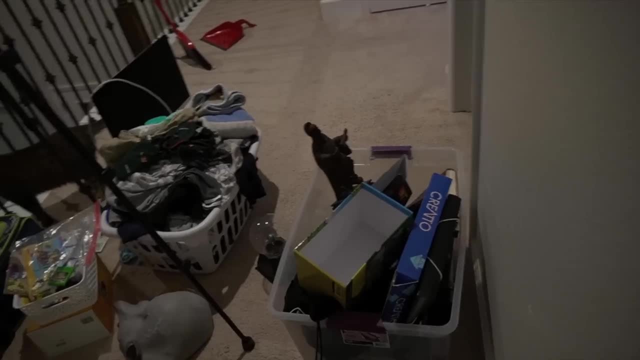 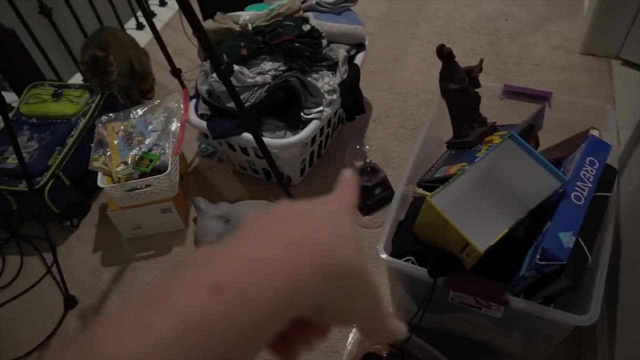 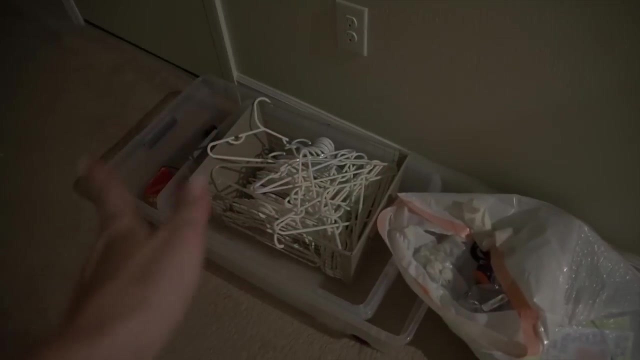 that we purchased to keep them busy, Like stuff from Hobby Lobby and like art pads and stuff like that Journals- It's not like really sentimental, That's broken, That's scary, That's trash, That's donate, That's dirty clothes, That's getting fixed Trash And you know you get the gist. 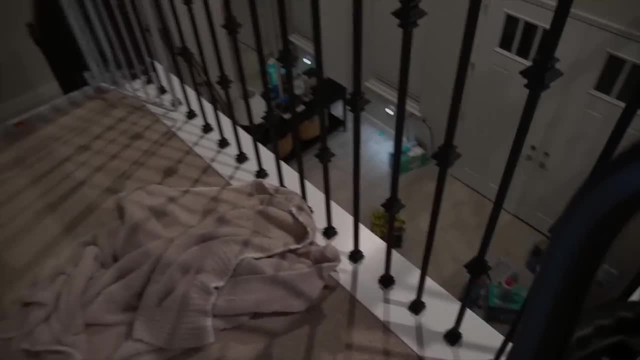 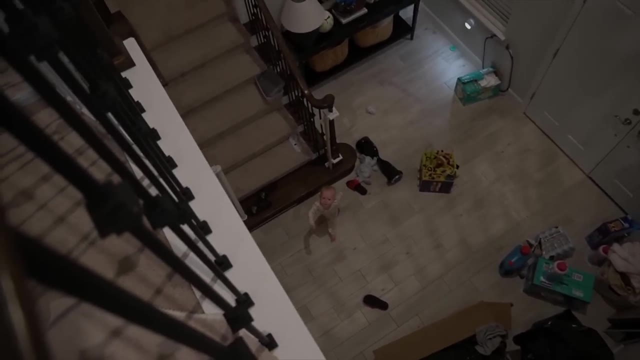 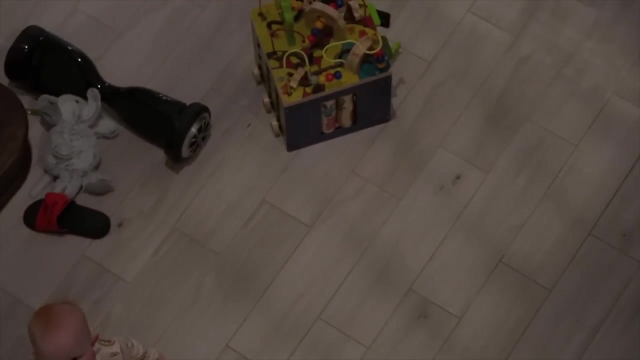 Pretty good. I think we've done really, really well. Um, I've done more and more laundry. There's Miss Emma down there, I'm coming. I've done more and more laundry And then I've even made a little pile out of the laundry that I've done, So it doesn't come up there. No point in it coming up. 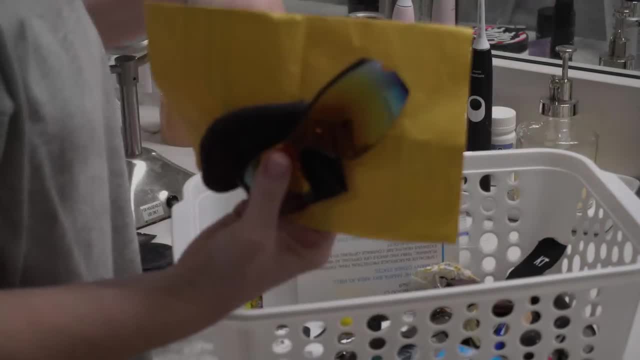 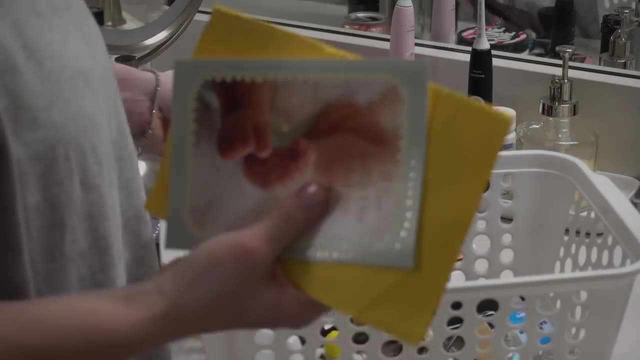 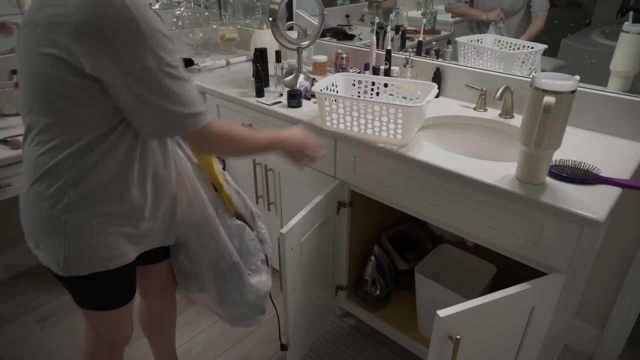 there Hi books. So I'm going to do a very quick run through of my bathroom. I actually filmed this a little while ago- It's probably it's been three weeks- and I wanted to just get in here while Emma was taking a bath one day and 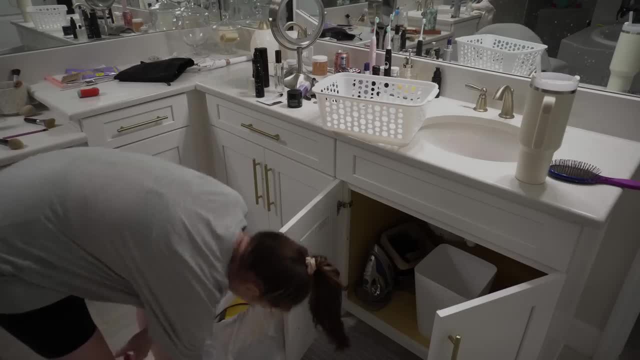 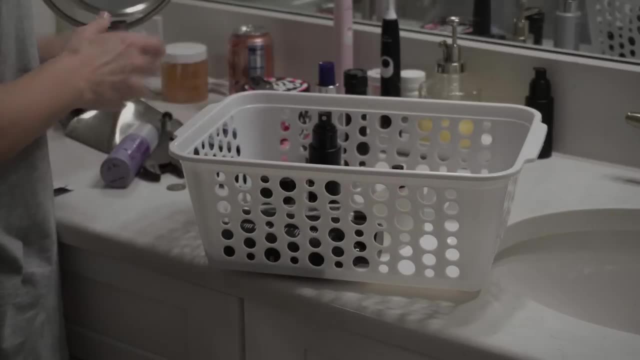 just clean it out And, like I had mentioned in so many other videos and even this one, start off with the trash. So anything that needed to be put in the trash makes it easy. My friend, my neighbor, loves dime and I love dime beauty as well, but I have invested in some pretty 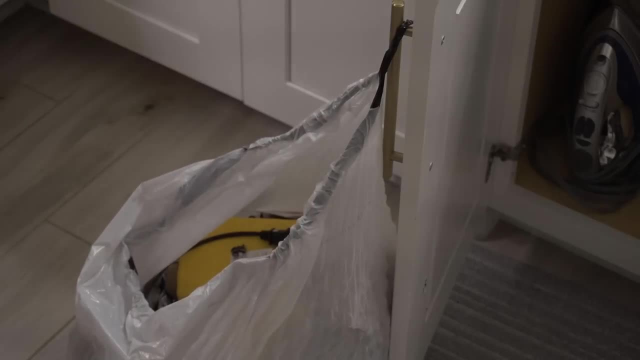 good skincare. So that was kind of like a little treat to myself when I turned 40. So I am going to be giving all of this to my neighbor. I'm going to be giving all of this to my neighbor. I'm going to. 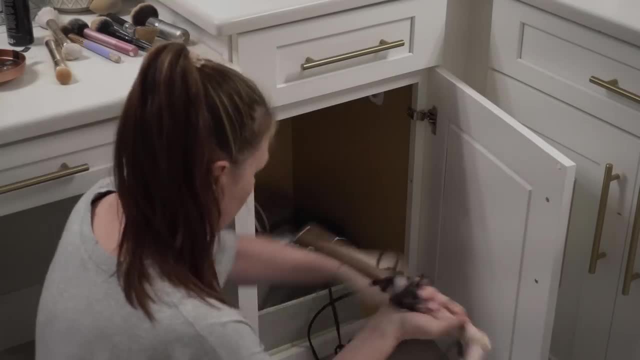 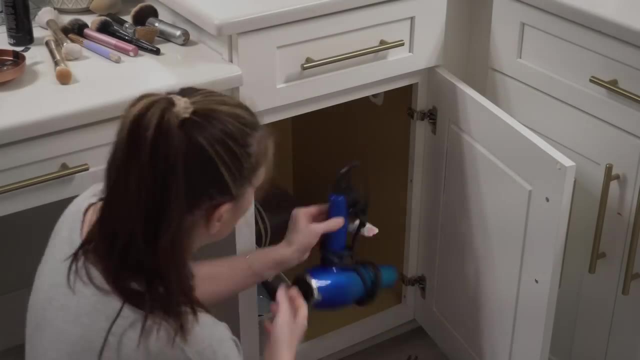 be giving all of the- well, not all of it, but the majority of my dime products- to her, because I have the other stuff that I'm using right now, that I'm using just every single day, And I don't want the other stuff to go bad, Not when somebody really wants it. So that's going to go to her. 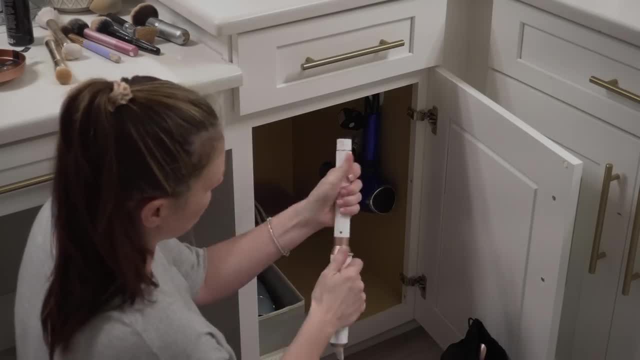 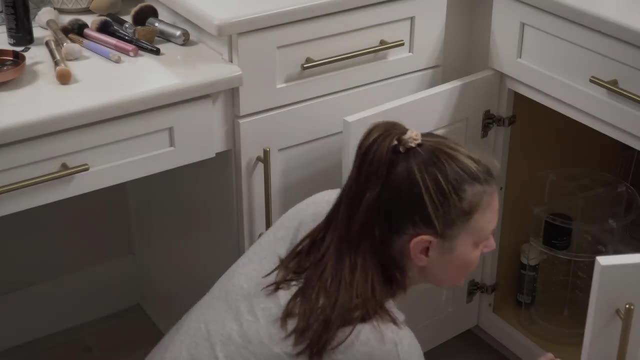 And then Chris got me this really amazing T3 curling iron that has, like certain heads you can take off of it. So it is everything I need. So I'm getting rid of all the curling irons- old blow dryers too, because he got me a new blow dryer for Christmas. 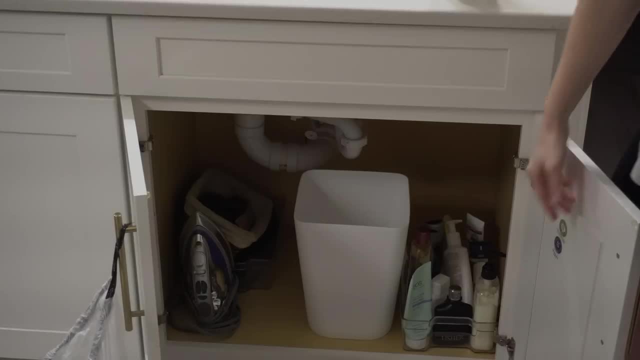 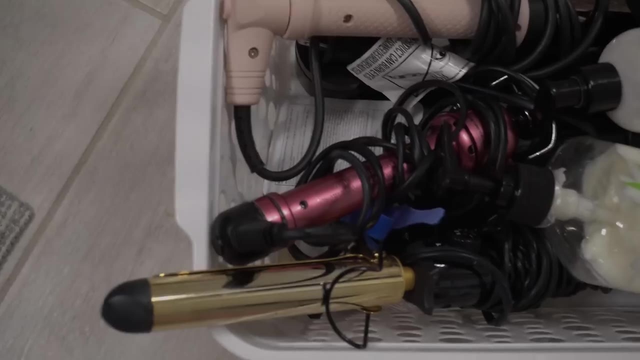 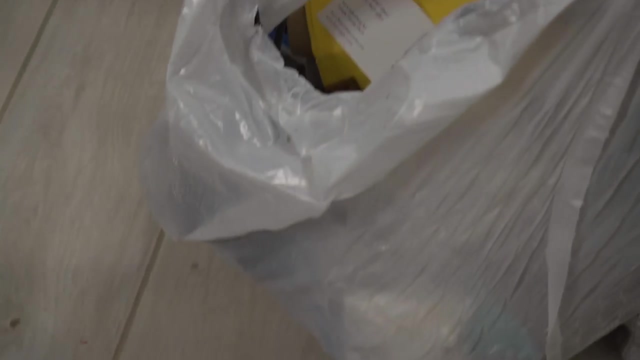 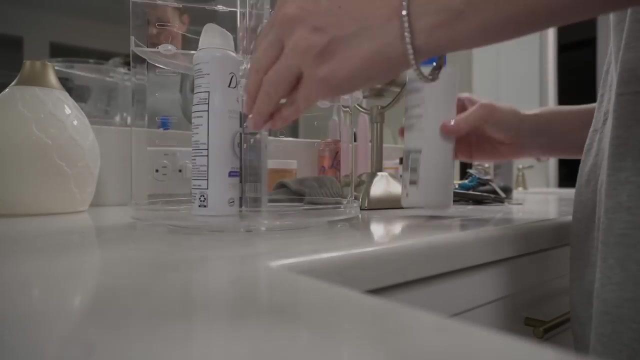 And then I'm going to go and also pull out some of the lotions and things like that. I am feeling so proud of myself for getting rid of so many things and having these bags here and just continuing to fill them up. It just feels so, so good. It's also helping me keep track of. where my money is going. So I'm going to go ahead and get rid of all of this. So I'm going to go ahead and get rid of all of this. So I'm going to go ahead and get rid of all of this. So I'm going. 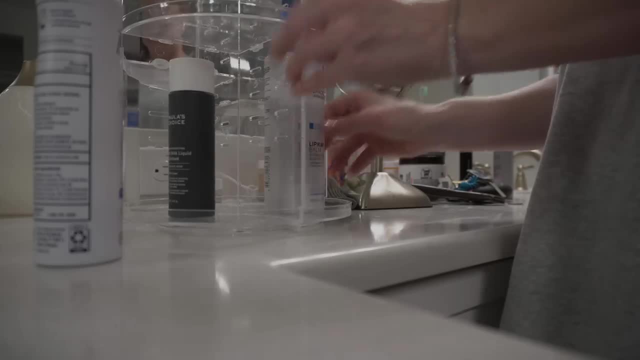 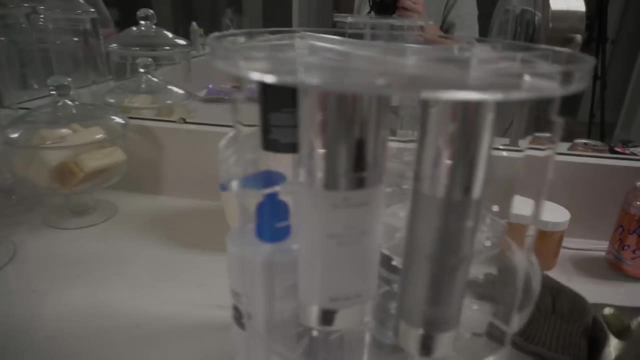 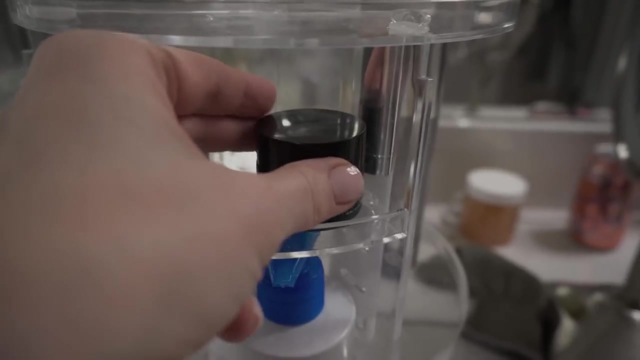 and I just realized I've wasted so much money. I spend a lot of money on things I've been influenced by. I think we could all relate things I don't need, And it has to stop. I have to stop bringing things into this house because it is overwhelming me. It is stealing my creativity. 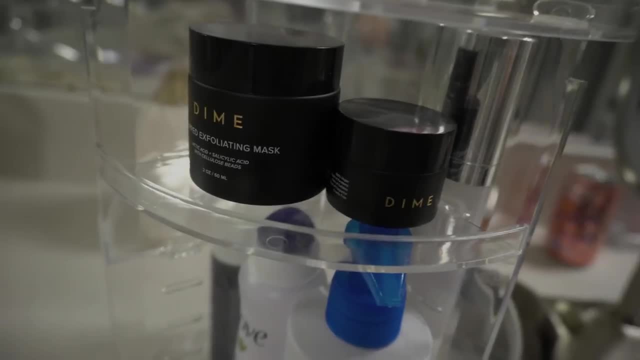 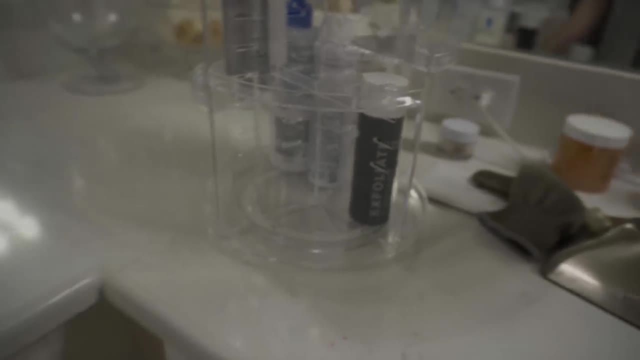 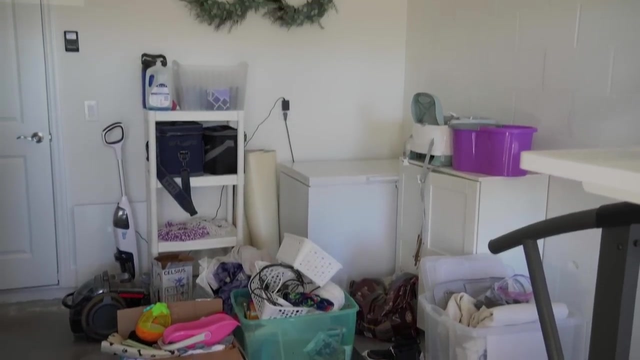 It is stealing my joy. It genuinely is. It is making me unhappy, It is making me unwell And we, we do not need to keep things that do not serve us. Even if someone gave it to us, we've got to let it go Now. I've got boxes in the garage here. As you see, I've been collecting. 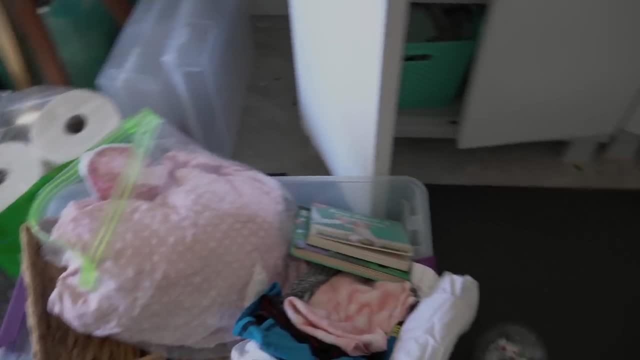 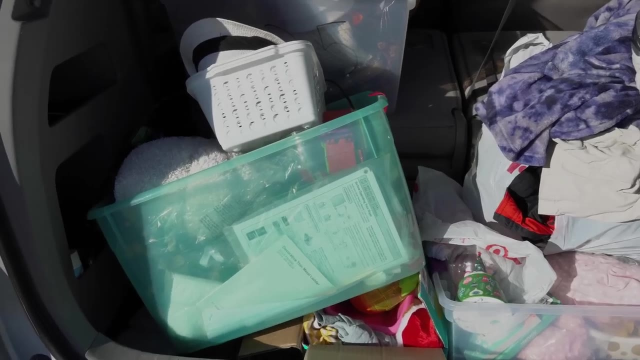 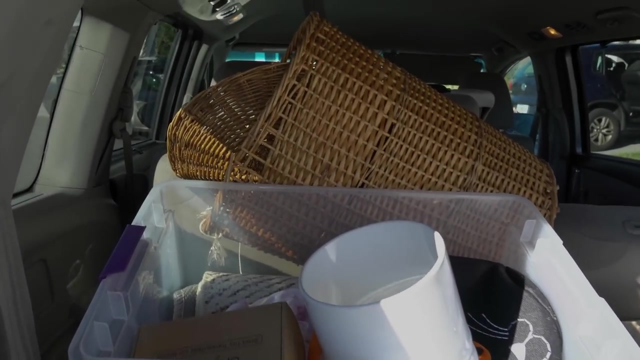 stuff. for a couple of months I have thrown things that I have come across in the garage And if I go back and get it, then maybe I needed it, But if I don't, I am taking it to the salvation army. So the cart is full and we are tackling this today. That is another thing. Be sure to get the